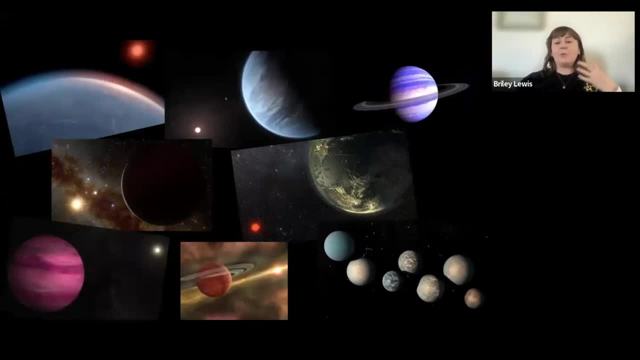 system, And so this makes sense. We are more familiar with the planets in our solar system, and the headlines about exoplanet results that are in the news often show us artist renditions. So these pictures that you see here are, all you know, ideas from artists. 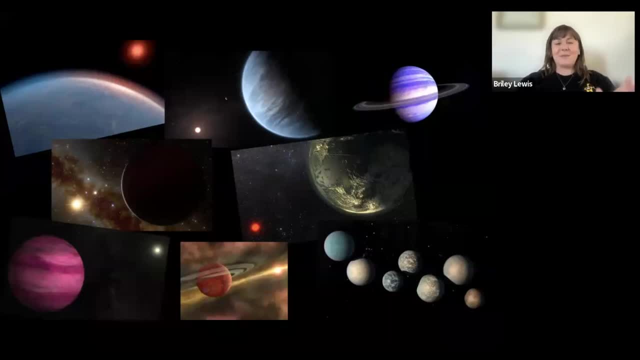 where they made up something that could be what it looks like, But it's a pretty picture, not actual data, And these are also often based on the children from viewers who actually off of our solar system, since those are the planets we actually have a really clear view of. 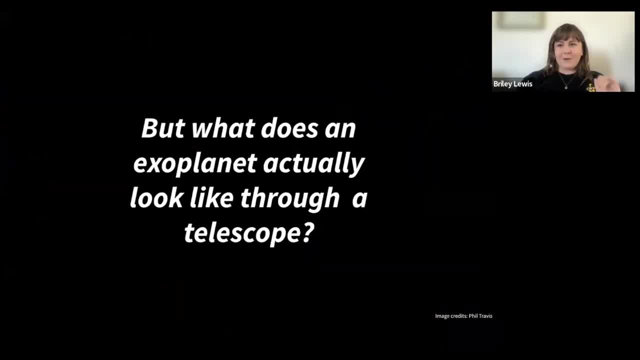 But what does an exoplanet actually look like through a telescope? And now here's where our first poll comes in. So question time. Kristen will put up the poll. What do you think it looks like? Your options are: maybe it looks kind of like Saturn or Jupiter through a backyard telescope. 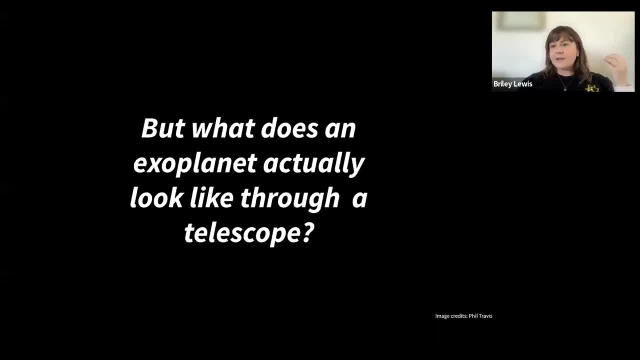 where you can see some of the- you know- stripes and the rings and everything. Maybe it looks like a fuzzy blob with some light and dark patches, Maybe it looks like just a couple of pixels in an image, or we can't see them at all. And I'm saying: what does it look like through a telescope? 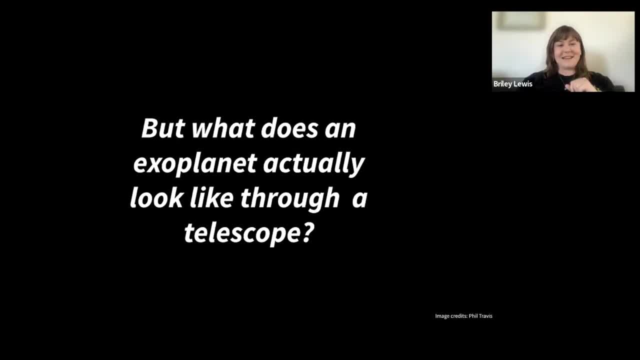 if you were trying to just take a picture of the planet, not collecting fancy data like light curves? Yeah, we'll give them a minute and the poll's running Ground, ice or space-based, doesn't matter. What do you think if we were to try to take a picture of an exoplanet? 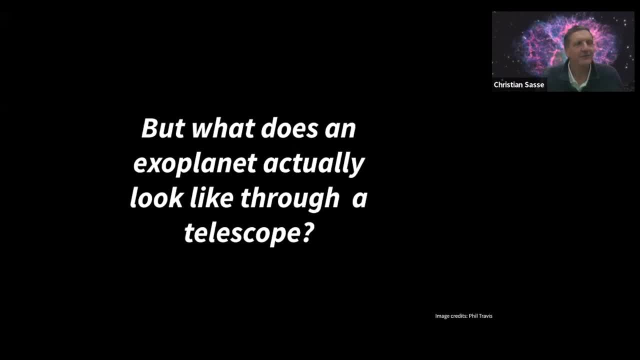 Okay, we'll give a few more seconds and then we'll share the results. I see a lot of people in the chat are thinking really hard about this one and thinking of all the ways we indirectly detect planets. But I mean if we were to try to capture light from the planet itself? 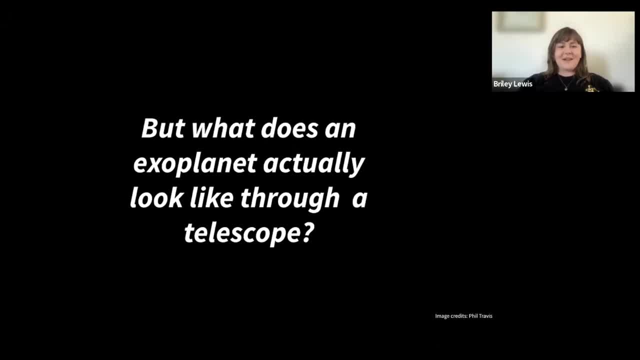 All right, we've got an interesting spread here, So we've got. 11 percent say kind of like the planets in our solar system, like we see them through backyard telescopes. 14 percent of people say a fuzzy blob with some light and dark patches. 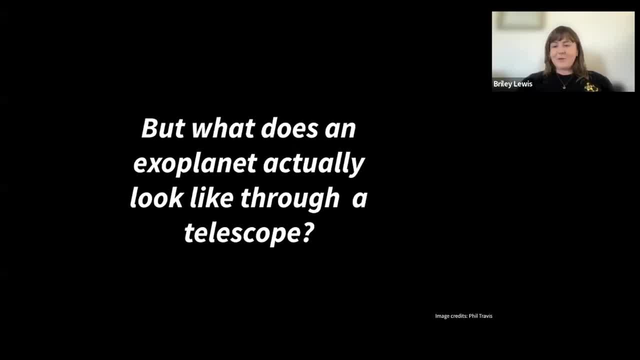 29 percent say a couple bright pictures in the image and almost half say we can't see them at all. well, I am super excited to prove you wrong and say that we actually can see them. So today I'm going to tell you about how we 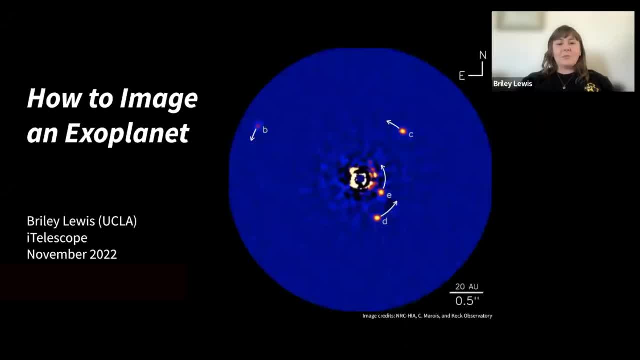 image, an exoplanet And people who said: a couple bright pixels in an image. you're spot-on. So the picture here is real data. This is the Hr 8799 system, which has four planets. I am other than the sun, US and the others, So the picture that we're taking, what we have here today, is the Hr 8799 system, which has four planets. 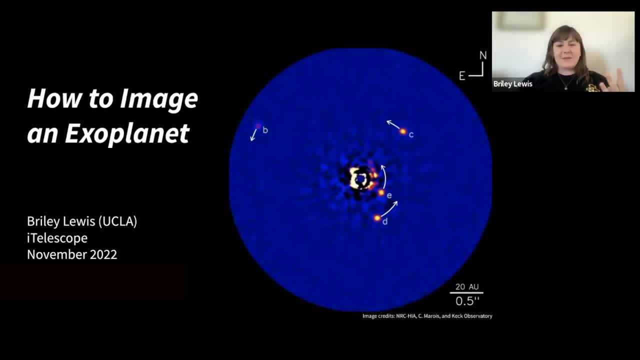 and it's labeled B, C, D and E in this image, And so this is what we're going to go into today: how we actually get data like this. Someone in the chat said maybe I could if I had a 10 plus meter telescope with adaptive optics. 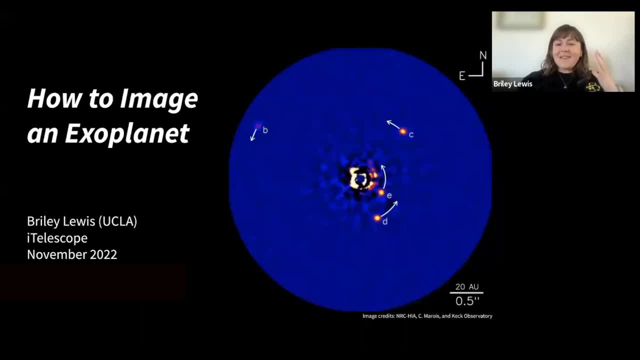 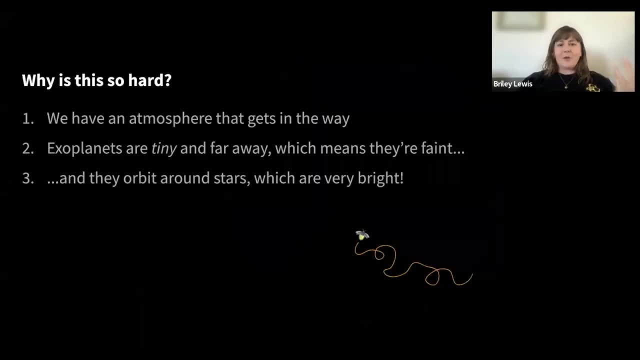 You are on the right track there, my friend. So these pictures can be taken, but they are very technically difficult. And so why is it so hard? There are three main factors. One: we have an atmosphere that gets in the way. 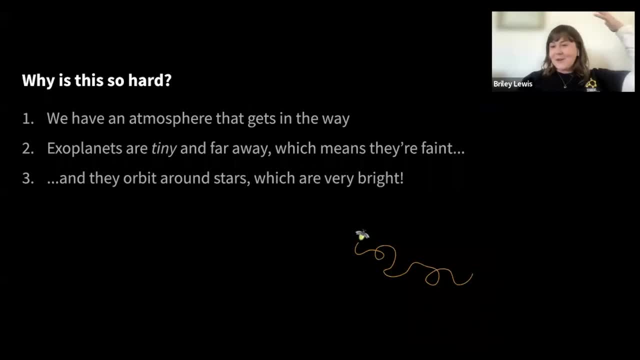 So the atmosphere of Earth, as you all probably know from observing, can get pretty lumpy, make your images blurry. That's the problem. And then the other thing that you can't get rid of just by going to space is that exoplanets 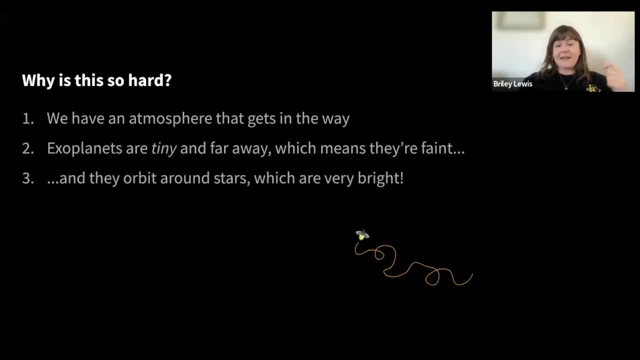 are tiny and far away, which means they are really really faint And they orbit around stars which are very bright. So you're trying to see a very faint thing next to a very bright thing, And so you can compare this to trying. 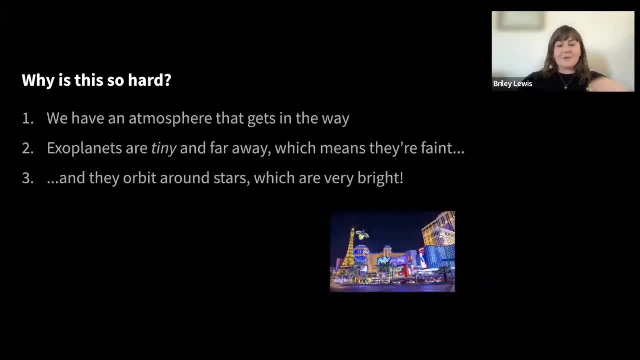 to take a picture of a Firefly that is buzzing around the bright lights of Las Vegas and taking that picture from here in Los Angeles. So you can imagine that is a very difficult thing to do. So let's tackle each of these problems one by one. 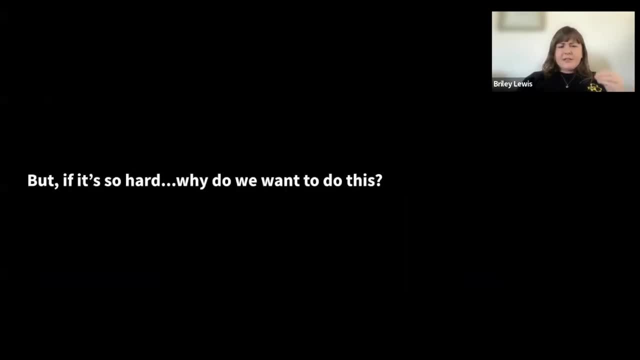 and how we can deal with them with technology. But first, if it's so hard, why do we want to do this? You guys already brought up in the chat: we have other ways of finding planets that we're really good at, So why are we trying to do this firefly around? 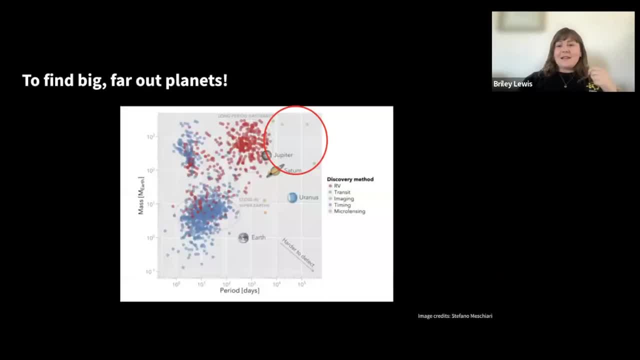 The Las Vegas lights nonsense. And the answer is that other methods of finding exoplanets can't see the same ones that we can see with direct imaging. So right now we're limited in technology by what each different method can find. So transits where you have the planet block out. 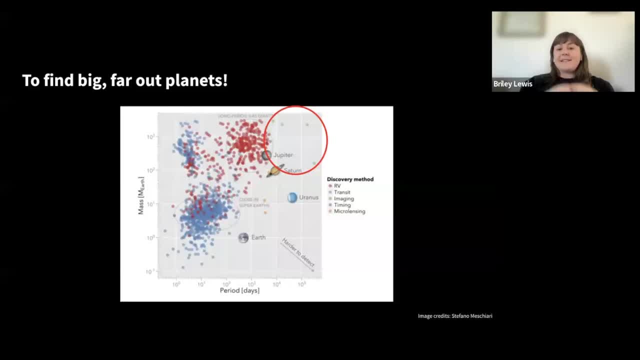 some of the light from the star as it passes across Transits are really good at seeing really close in big planets. So our radial velocities where you see shifts in the planet's spectrum And imaging is uniquely good at getting these far out very big. 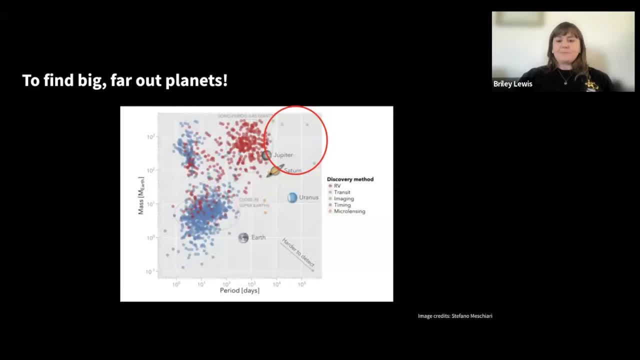 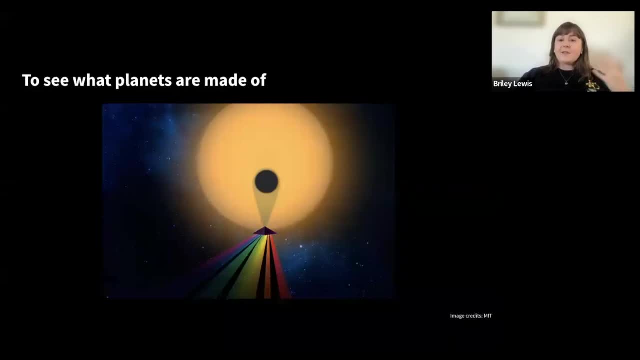 planets, so the outer gas giants in a system, And the other thing is we want to see what planets are made of. So there's a couple of ways of getting spectra which can tell us about composition, And one of those is by doing direct imaging. 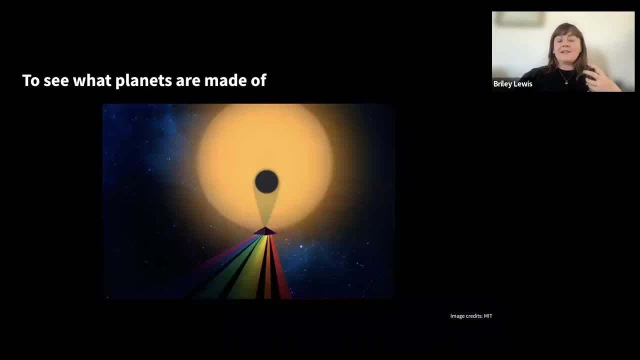 where you're actually getting light from the planet itself And the spectra we can get from direct imaging, you know, can tell us about what the atmosphere is made of, and more, And as this technology improves, it's what we hope will be able to tell us. 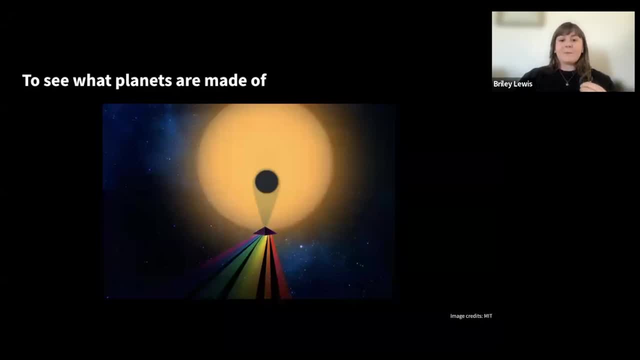 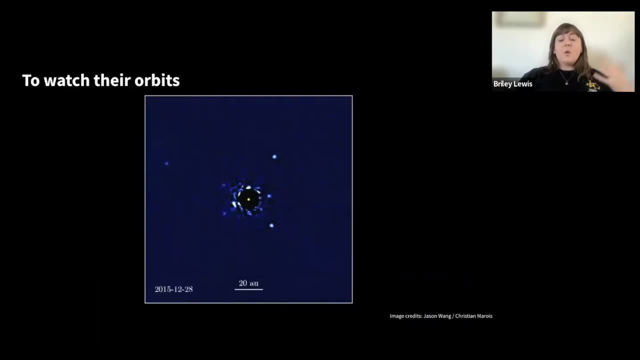 about habitability and signs of life on other planets. And the other cool thing about direct imaging is that we can actually watch the orbits of these planets. So, unlike other methods where you have to disentangle these different signals, with direct imaging you can just actually watch them move. 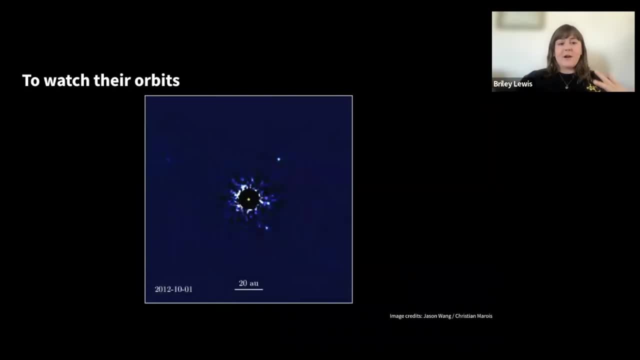 So this is again the HR 8799 system, And it's a very powerful system. It's a very powerful system. It's a very powerful system that we saw on the first slide. These are infrared images taken by the Keck telescope in Hawaii. 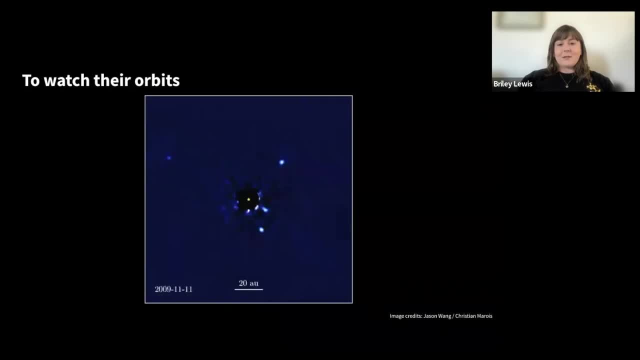 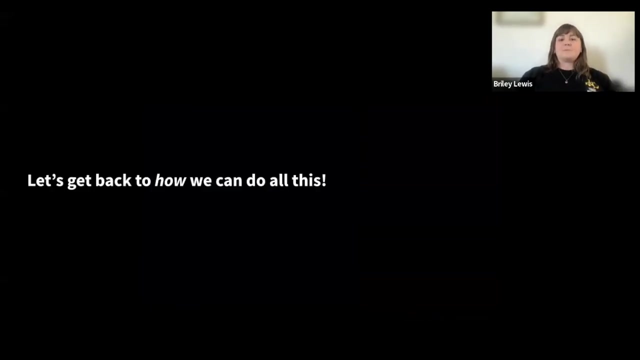 And you can see how, over the years that this system was observed, those planets are clearly moving in their orbits, So we can actually just watch where the four different planets are. So now that we've got some motivation, let's get back to how we actually can do all of this. 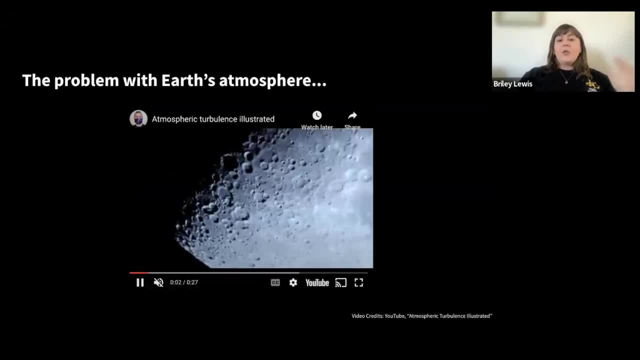 So first we're going to talk about the problem with Earth's atmosphere. Although now we do have some space based observatories that can do direct imaging, like the James Webb Space Telescope, we're going to focus on direct imaging from the ground. 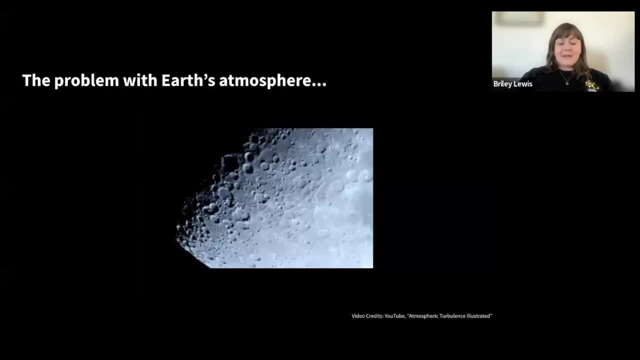 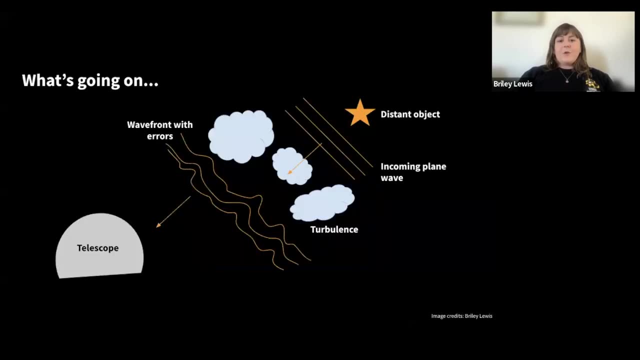 because that's, admittedly what I personally work on and something that's going to be very useful in the next few decades. So the problem with Earth's atmosphere is turbulence. So what's going on in the atmosphere? We've got a distant object like a star. 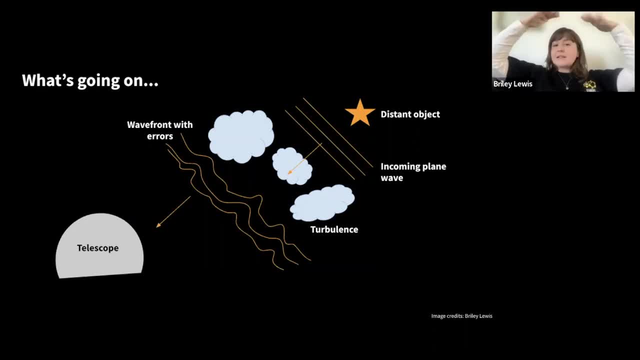 with a planet around it And as the light comes into the atmosphere, it's this nice flat plane wave of light, But then it hits the lumps of our atmosphere where there's different pockets of air at different temperatures and they 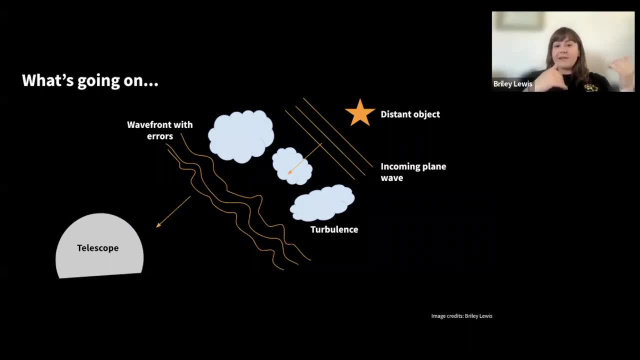 change the index of refraction of the light, so how much the light bends. And from this nice plane wave going through all those different lumps and bumps of temperature in the atmosphere, you end up with a wavefront of light that has all these bumps and wiggles in it. 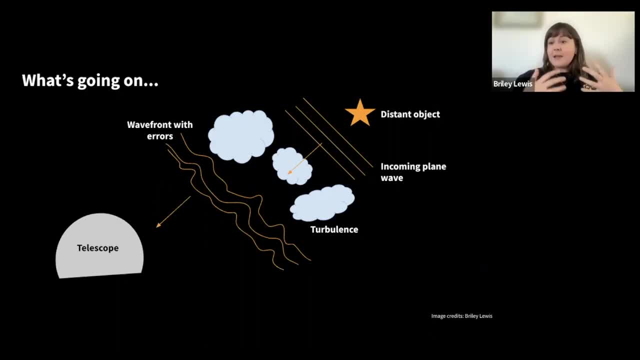 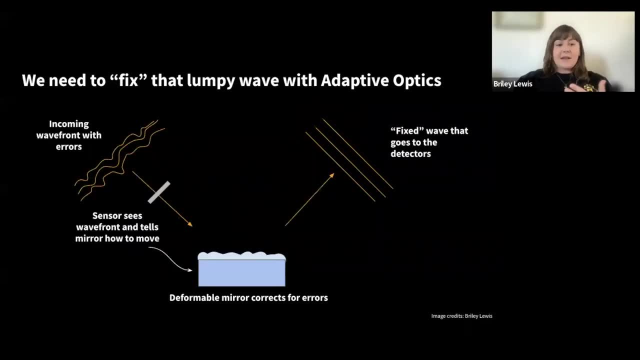 And that's what creates the blurry images that you see on a night with really bad seeing. So that's what's going on in the atmosphere and we need to correct it. Someone already said adaptive optics. That's exactly what we use here on the ground. 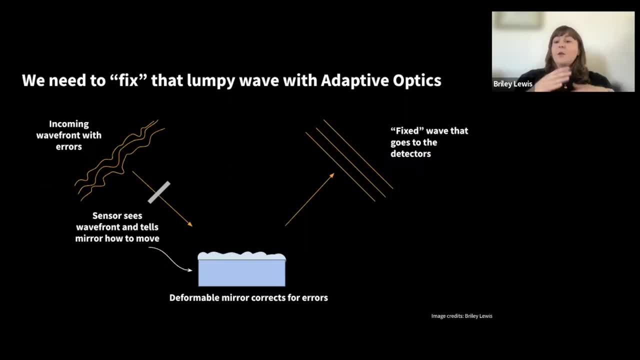 to correct it nowadays. So for adaptive optics, that's how we fix these lumpy wavefronts. You've got an incoming wavefront with all those airs and then a sensor that looks at that wavefront and tells a mirror how to move. 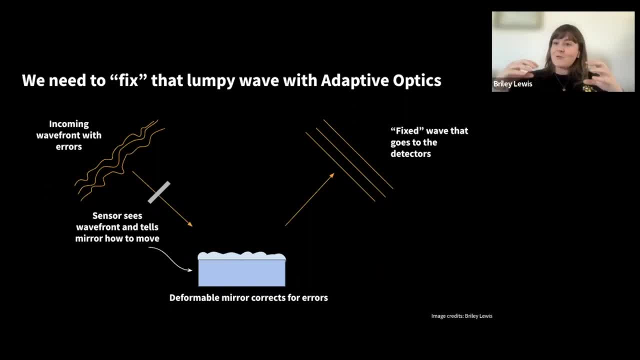 And then that deformable mirror, so a mirror that can actually change in shape, corrects for those airs and you get it back something at least kind of close to a fixed way. that's all nice and flat. that then goes to your detectors. So we're basically correcting for all the errors of the atmosphere with this flexible. 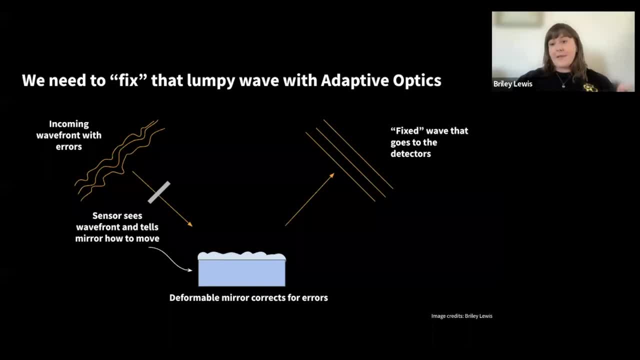 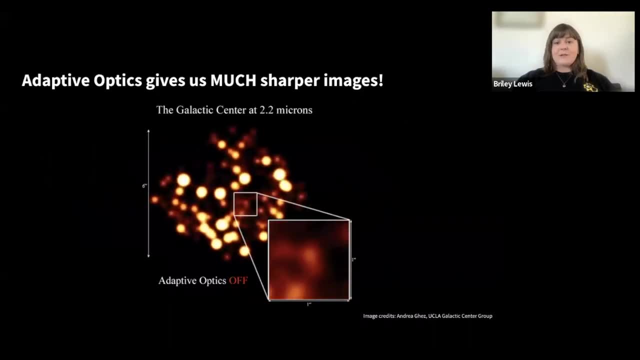 mirror And adaptive optics can do awesome things. I bet a lot of you know about this already, but adaptive optics gives us much, much, much sharper images. So this is an example from one of the groups here at UCLA that studies the galactic center with Keck, and it's a gif that's. 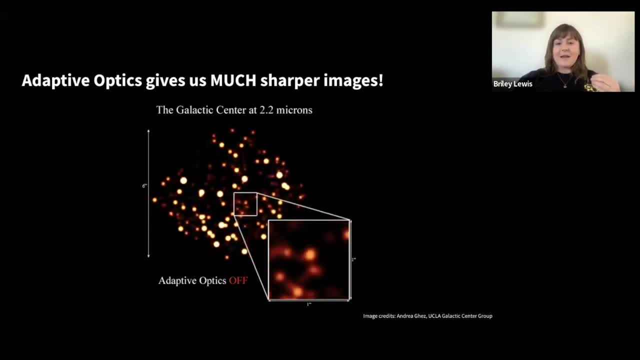 flipping between what the galactic center looks like in infrared- without adaptive optics we can see it's very blurry- and then with adaptive optics, where you can resolve a bunch more stars than you could otherwise and they're clearer, sharper points of light. This is a really big difference and 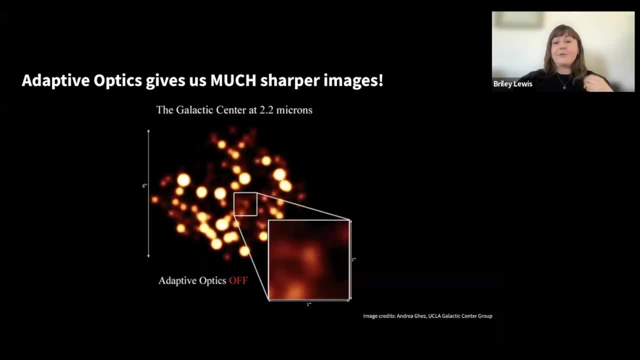 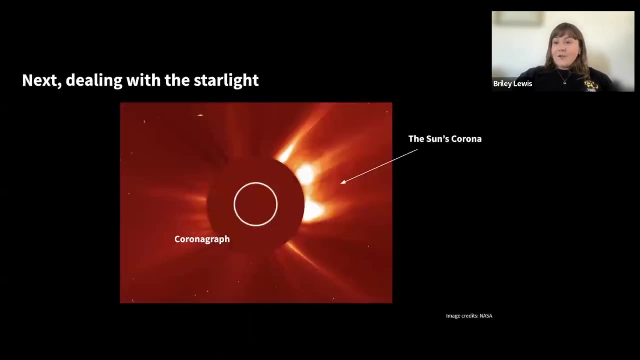 that's something we have to do in able to in order to be able to have crisp enough images to see those tiny, faint planets and resolve them from their star. So adaptive optics- step one works really well. We're pretty good at this nowadays, And so the next step is dealing with the starlight. So the star is. 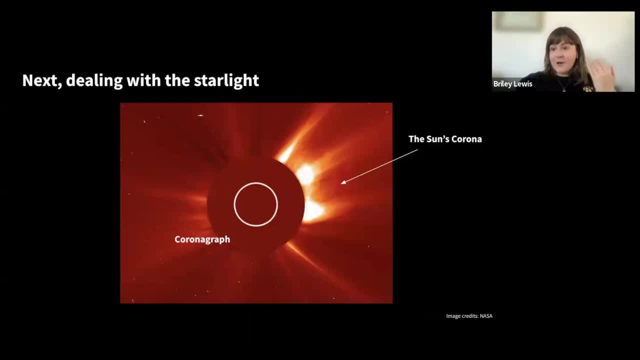 bright, the planet is very faint. We call that having a high contrast between the two things. So what we use is a little tiny piece in the optics called a coronagraph. These were originally designed for use for the sun, where you would take this little sort of black dot block out the sun. 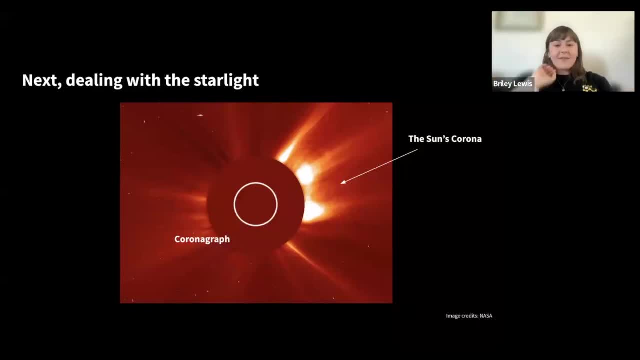 and then you'd be able to see the sun's faint or corona around it, like in this picture. You can kind of also think of this as if you're standing on a stage with really bright lights and you can't see the audience in front of you If you put your hand up to block the lights. 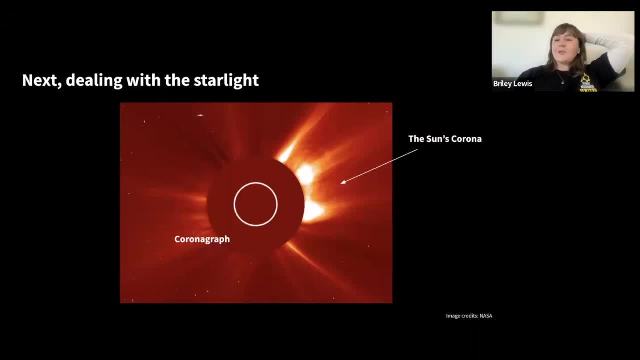 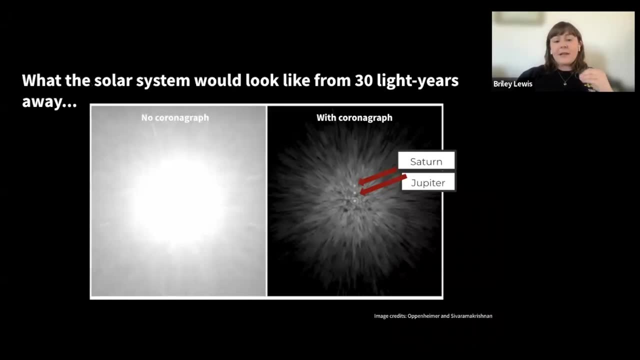 then you'll be able to see the fainter audience, since the bright light isn't shining in your eye. So it's the same principle, And coronagraphs are extremely important in being able to image planets like this. So the picture on the screen here shows a simulation of what, the corona of what 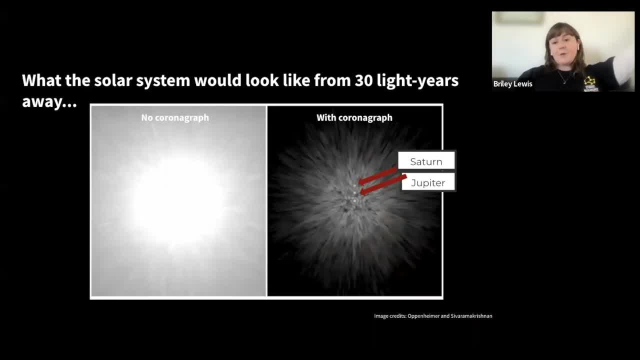 solar system. our solar system would look like to an observer 30 light years away from us And on the left there's what it would look like without a coronagraph, where all you see is the bright glare of the sun, And then, with a perfect coronagraph, you'd be able to see things like 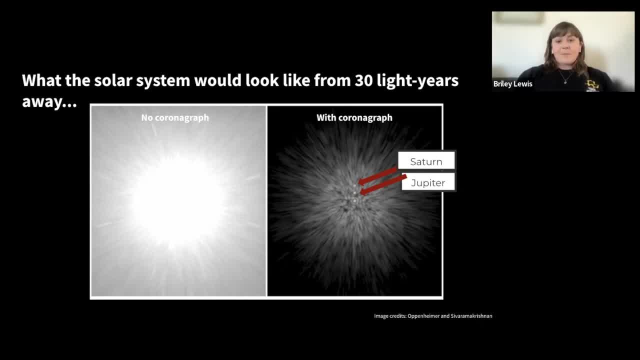 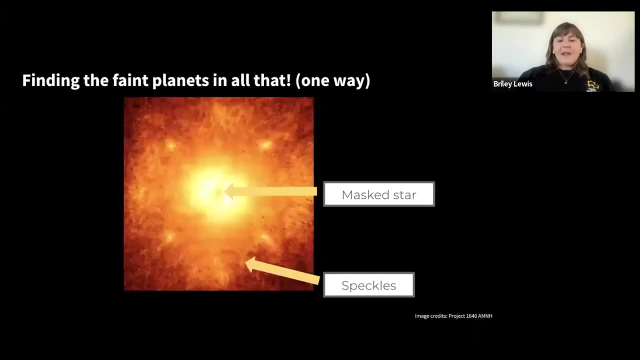 Saturn and Jupiter clearly showing up as little dots. So blocking out the sun is the difference between seeing nothing and clearly seeing Saturn and Jupiter. So this is a huge part of our system is the coronagraph, And then we have to actually find the faint little planets. in all, 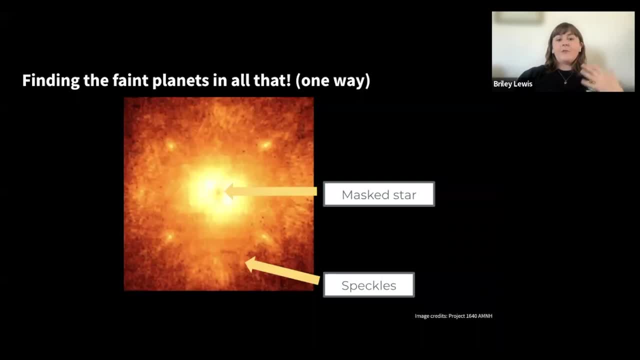 of this. So this is what some of the data looks like from these kind of direct imaging systems here on the ground before we do all of our data processing. So one way of finding faint planets- and I think this gif isn't working. This is supposed to be a gif, So this should be a video. 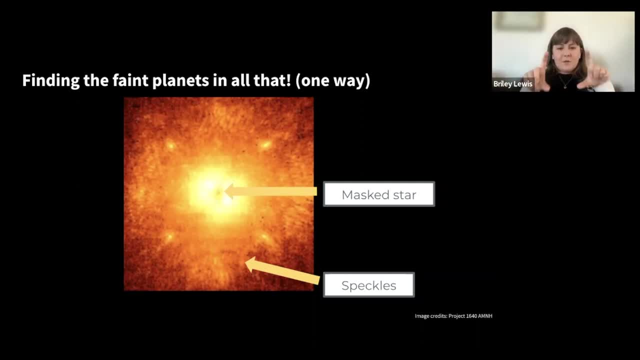 where each frame is a different gif. So I'm going to go ahead and show you how to do that. So the first thing is to find the faint little planets that are moving in different wavelengths of light, And what you would see is those little speckles that make a square, those little dots. 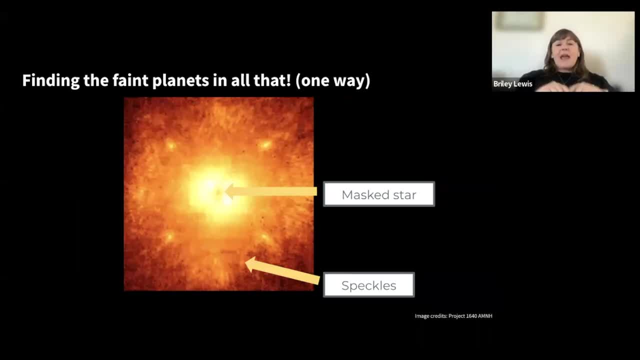 Those will actually move out with wavelength And that's just a feature, like from diffraction of light. So just because at different wavelengths the light is bouncing up the telescope a little bit different, your things move out. But planets and real objects out in space don't behave like. 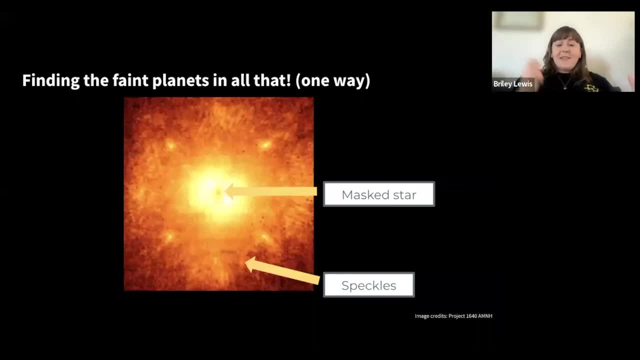 that They stay in the same spot, And so that's actually one of the ways that we can can differentiate, OK, what is just a little dot of noise and what is a planet. This is called spectral differential imaging. There's a couple of different ways. 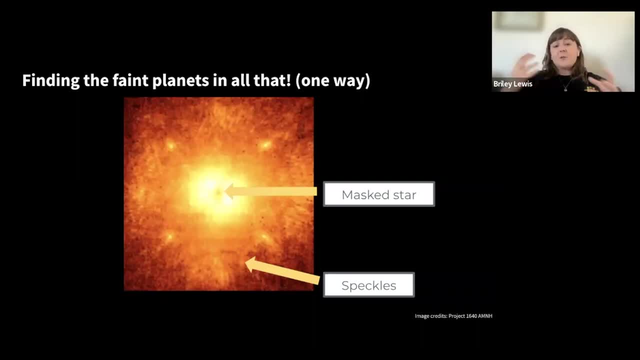 that we can find faint planets in our data reductions besides this, but I'm not going to go into them right now. If you're curious, we can talk about that later. So if we were to be able to see this moving, you would see that there's fairly clearly. 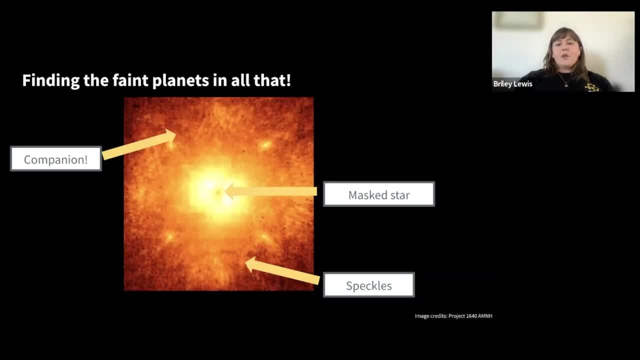 once everything's moving a little dot right here, that stays still. So this is actually not a discovered planet. Hilariously, I say it's a companion because people thought it might be something, but it turns out it was actually a background star. 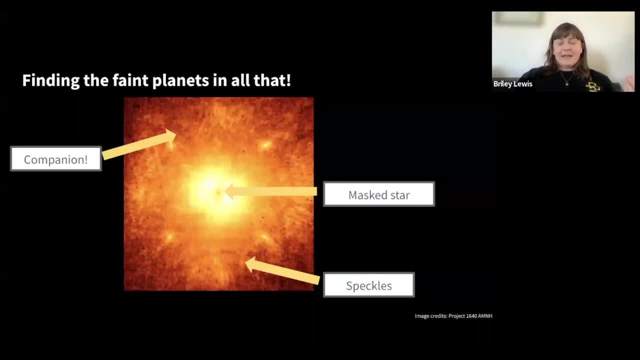 But the point here is, in order to actually see faint planets, we need to do some kind of data processing, So we need to get rid of all the extra noise that is still left over after the adaptive optics and the coronagraph, And so when you take out the rest of those speckles, 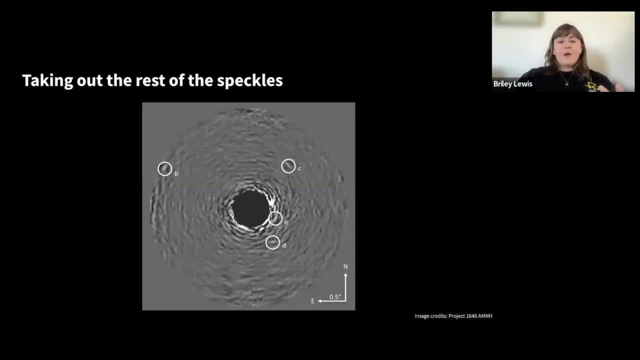 you get an image like this where you can actually see: OK, there are real planets that were hidden in that noise. So what we do is we use the data itself to make a model of the noise and then subtract that from the image. So if you have an image that is signal plus noise, 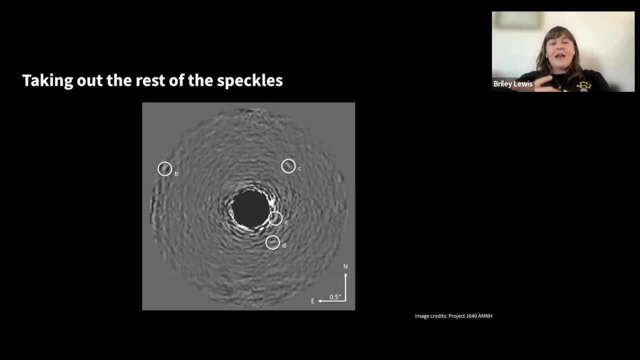 and you subtract the noise. you should just have your signal after. And so if we make a model of these speckles, the speckle noise, and then subtract that out, we should get our planet. And that's what you see here. 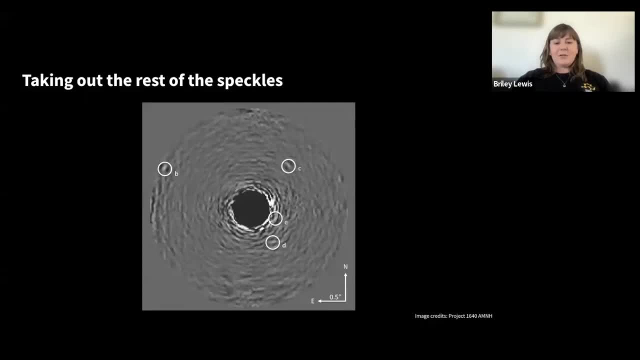 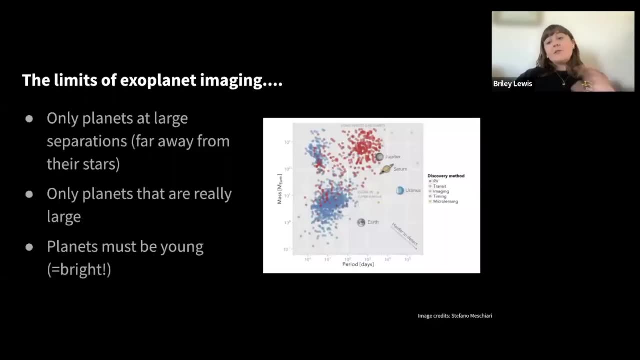 This is again a different view of the HR 8799 system we've been looking at so far. So there are definitely some limits to this technique though, just like there are to the other techniques for finding exoplanets, like transits and radial velocities. 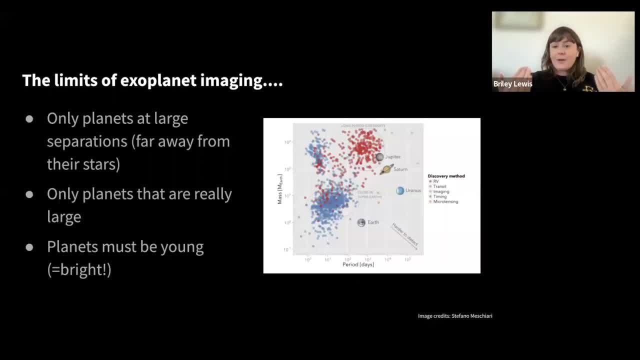 So everyone has their advantages, but everyone also has their limitations right now, which will hopefully not be as strict as we improve technology. So right now, Direct imaging can only find planets that are at large separation, so meaning they're far away from their stars. This is because the closer in you are to the star, the easier it is for the planet to get lost in the bright glare of the star. And also, if we're blocking out the star and something's right next to it, we might block out that very close-in planet. 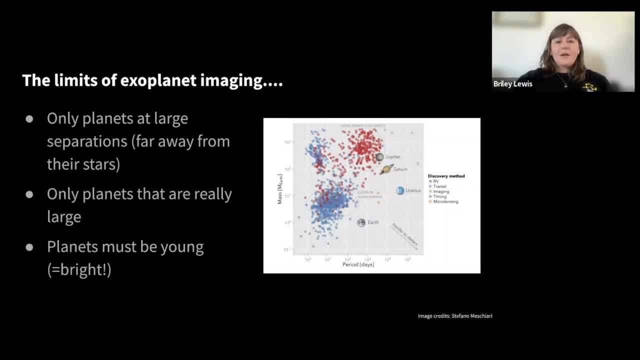 with the coronagraph. So, oh, I see a question, I will answer that one. So is there really a physical object in a coronagraph? How big would it be If? by physical object do you mean like, is it actually like a little spot that is blocking it out? 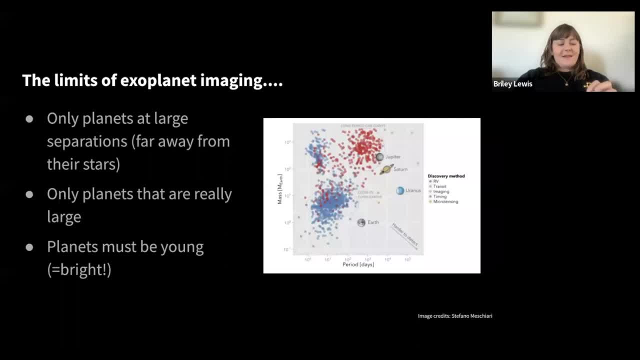 like a physical thing. The answer is yes. The masks are usually not actually just a black dot in the center where the star is. It's the opposite, where it reflects back everything besides the starlight And there's actually just a hole in the center of a mirror. 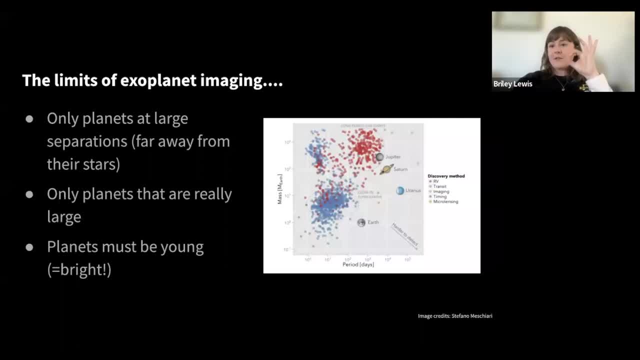 But they are actually about the size that I'm holding up with my hand right now. for a lot of things They're very small Because what happens is you take the big beam of light from the telescope and then you focus it down to go through the optics of your instrument. 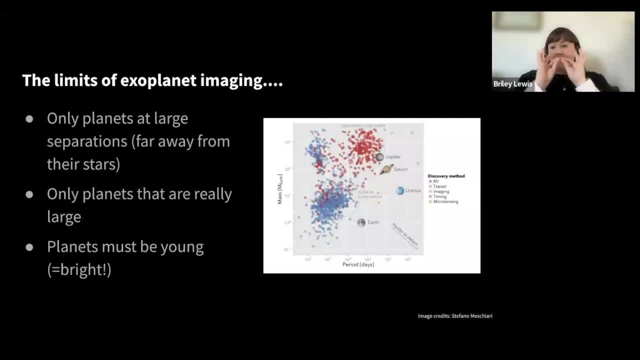 So they're not very big, They're pretty small And the hole is even smaller, Absolutely tiny. So I hope that answers your question. So back to our limits and advantages. Our limit: we can only see planets that are far away from their stars. 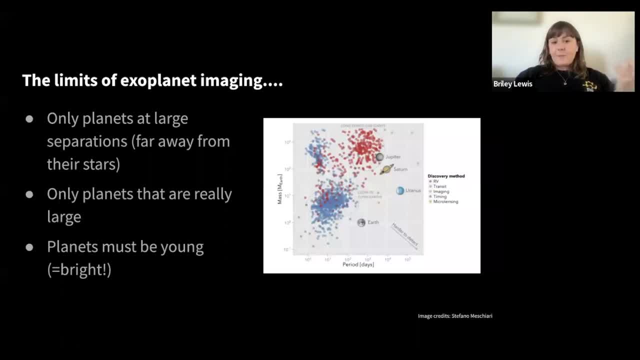 because of that bright glare of the star closer in- And this is something that people are really actively working on- trying to improve how close we can see into the star with better instrumentation. Right now we can also only see planets that are really large. 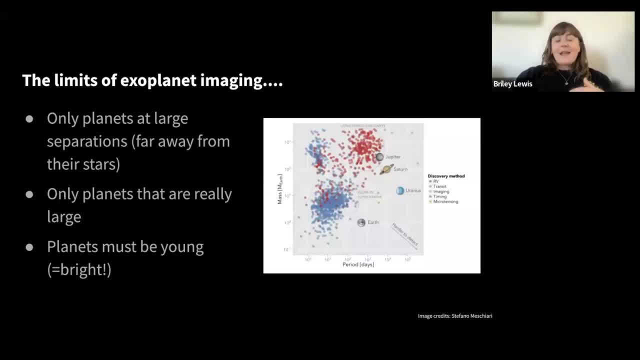 So a bigger thing is going to emit more light, And so that is something that we're currently limited by, because we need to see something bright enough to make it beyond that glare of the star, And, again, this is something people are really working on. 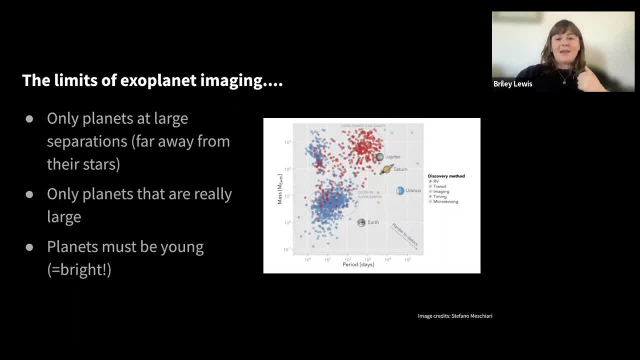 trying to find smaller things. So I hope that answers your question And this is something we're working on. So we're working on a whole system of solar systems that does not emit as much rays of light as what we're seeing. So we're working on a whole system. 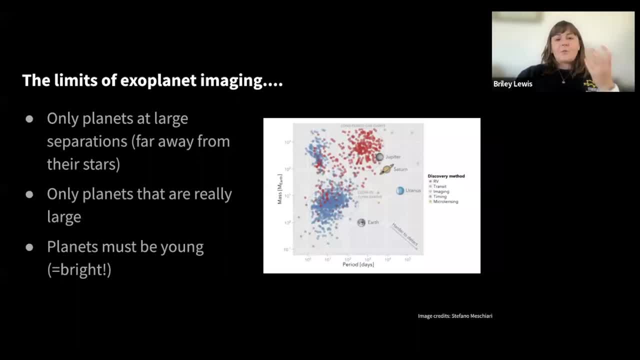 that does not emit as much light as what the Moon is, but instead we're looking at what we're seeing. So then we can also have the image of the sun and the stars in the sun, and let's see what the lights look like. 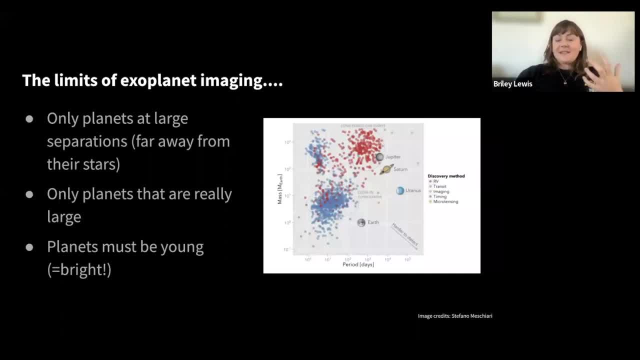 The image of the sun is outside the sun and it's looking like the sun has become much brighter. So you might get a little bit of a sort of latinx imitation of something Like the sun is moving so fast. And then the other thing. that's a really interesting caveat. 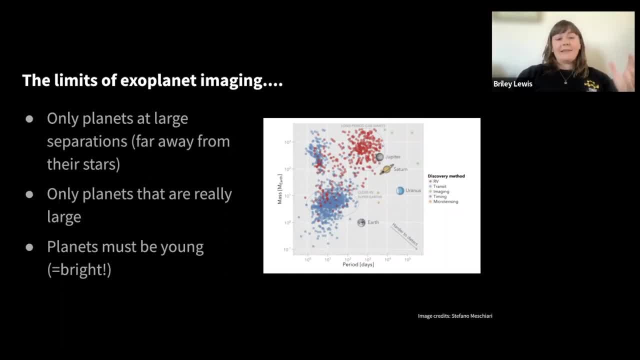 for exoplanet imaging is that the planets have to be young, so they have to have recently formed from the star. right now We're looking at infrared light, the heat from a planet as it just recently formed. So when a planet forms, you know there's a bunch of things coalescing and that leaves a lot. 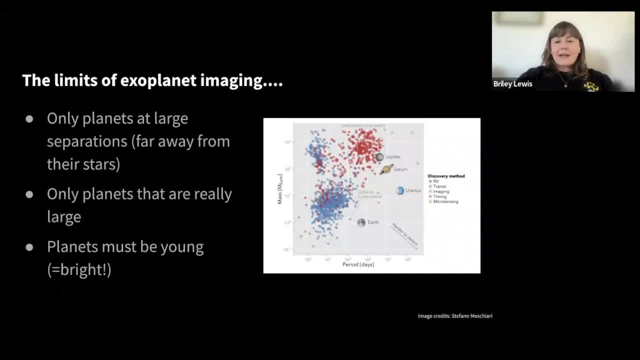 of heat from all these things that have collided together to create a planet, And so when planets are young, they are actually what we call self-luminous, So they are emitting a lot of light themselves, And so right now, direct imaging generally looks for planets that are really young. 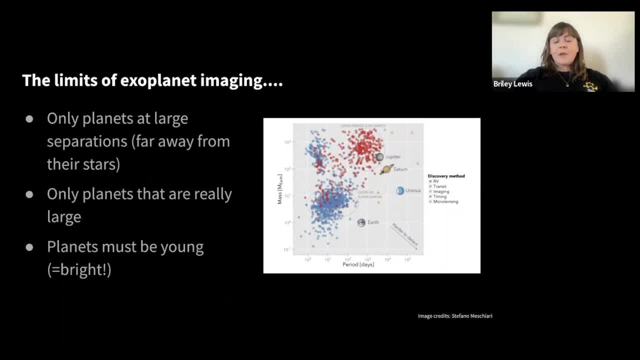 because those are the ones that are brighter- haven't cooled off yet. So that is another interesting limitation of this technique. right now I got a question of: can you please explain the third point? I think that's what I just explained, So I think you may have gotten a. 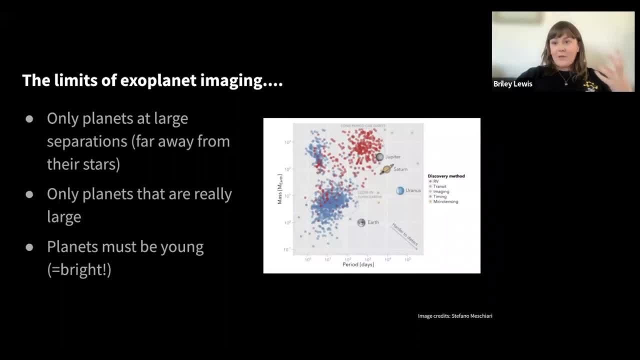 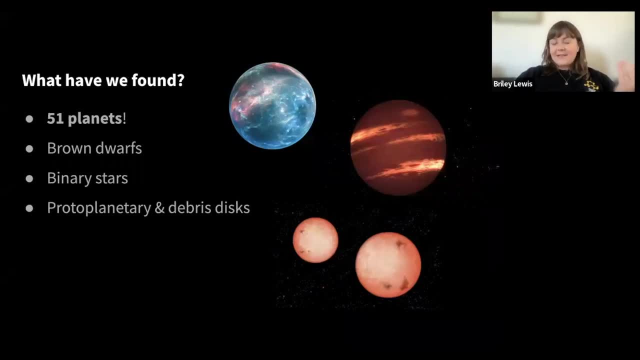 little ahead of me, but pretty much they must be young, because they're brighter when they're young. So what have we found so far? We've found 51 planets. I think this number has actually gone up to 52 or 53.. 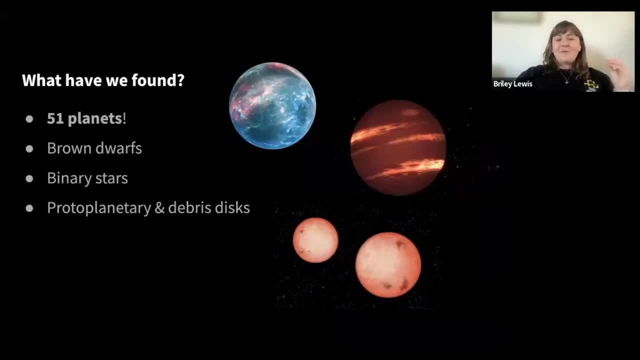 But there's a little debate. It's around 50.. We've also found some brown dwarfs, which I'll talk about what those are in a second, Some binary stars, so two stars orbiting each other And then a lot of. 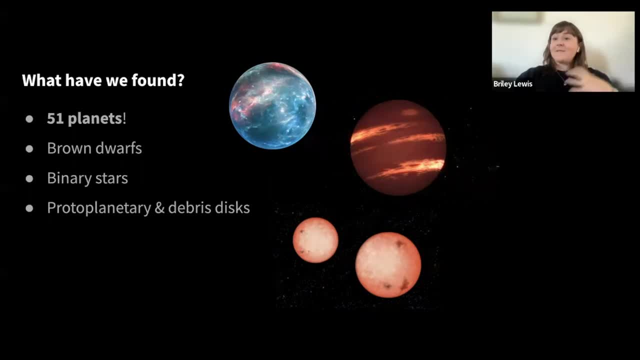 protoplanetary and debris disks, so the disks of gas and dust that are making planets. I've got a question again. I'll answer that one. So if the planet is young and hot, doesn't that also mean there's probably still a lot of debris around the star? But wouldn't the debris interfere with the? 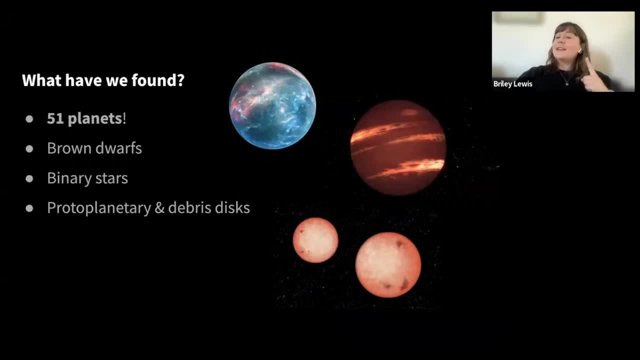 IR signal from the planet. Ooh, that's really interesting And we're going to get to some pictures later that, I think, will tell you that. So we've seen a lot of planets where the debris has been cleared, but we've also seen ones. 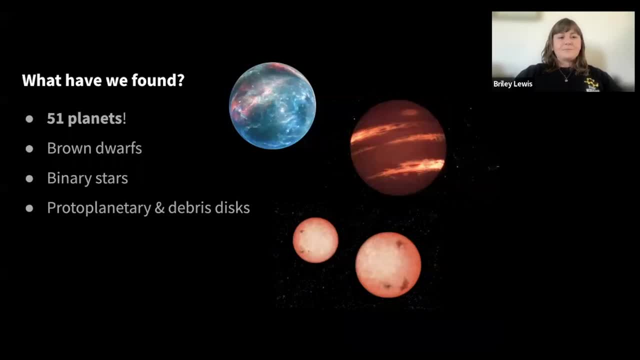 where it hasn't, And I will show you some pictures of that later. All right, So, Christian, can we put up our second question? So, just out of curiosity, what would be the most exciting thing to find around another star? to you, Would it be an exoplanet that looks like Earth? 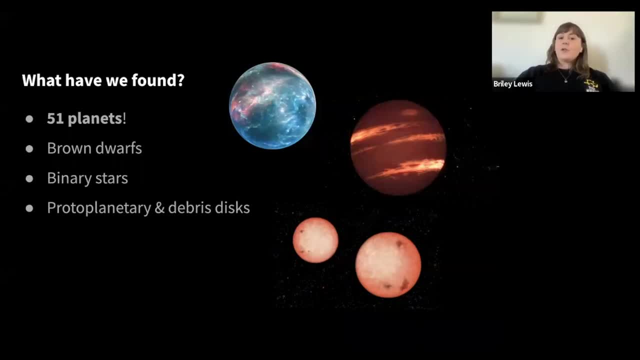 Would it be a black hole, another star like these binary stars, or something that's technological, that wouldn't occur in nature? Oh, I see in the chat an exomoon. That's a fun one. Oh, this is going to be an interesting one. I'm curious to see. 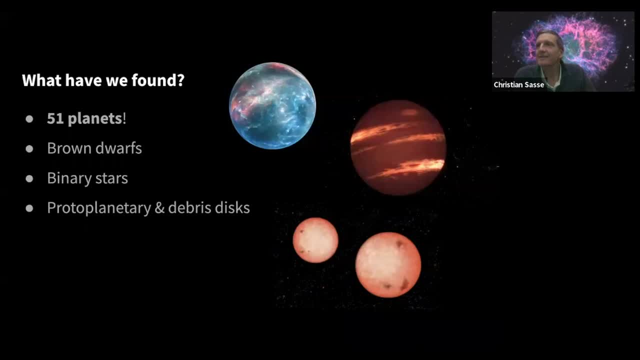 Well, this pans out. What do you think, Ronnie? Okay, So you know, that's actually about what I expected, honestly. So, Earth-like exoplanet- yeah, of course that would be exciting. That might have life, A space station or something- technology that would. 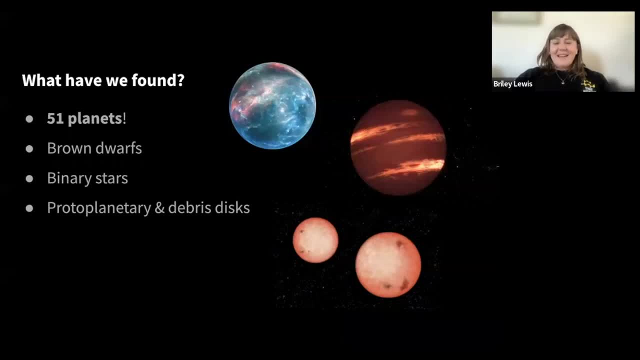 also mean you know, there must be something that created it, And then a couple people are interested in a black hole. I think that would be really cool, Like it would be weird, Like how did this black hole get to be orbiting? 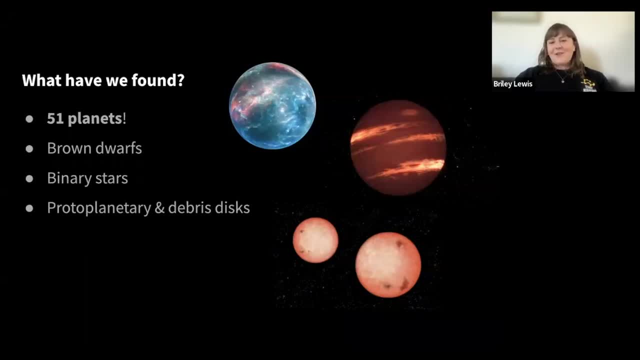 This little star And then another star. So I guess we're not very interested in binary stars here, but they can actually. they're very interesting scientifically, So we still try to try to find them when we can. Okay, So these are the things we've found, And if you're ever curious about getting a very up-to-date count, you can. 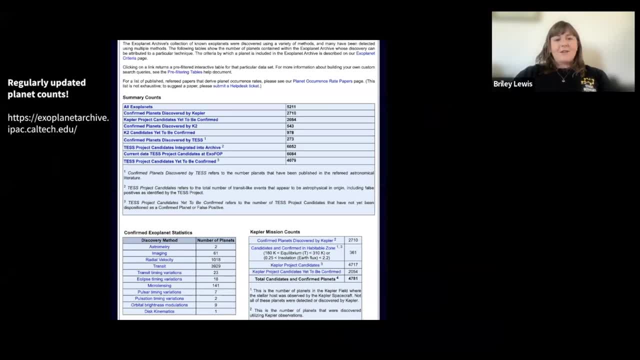 go to NASA's exoplanet archive. I put the link up here. This is how you can check up on the number of planets we've discovered, And they even sort it By what method they were discovered with. So right now it says 61 planets with imaging. 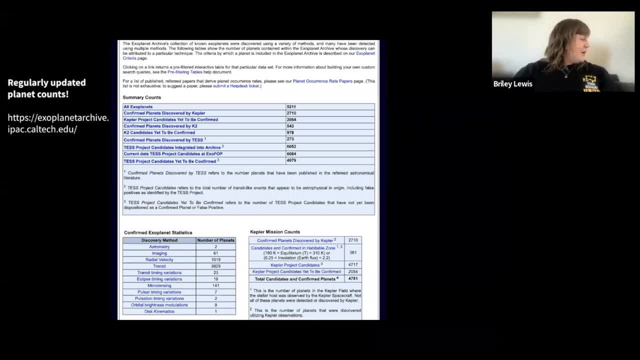 But again, some of them are kind of debated. still, I know this is a little small. I tried to get a screenshot just to give you an idea of what this looks like. And so right now we have discovered- and I pulled this picture yesterday, So as of yesterday, we've discovered- 5,211 exoplanets, And a lot of those were from the Kepler and TESS missions. 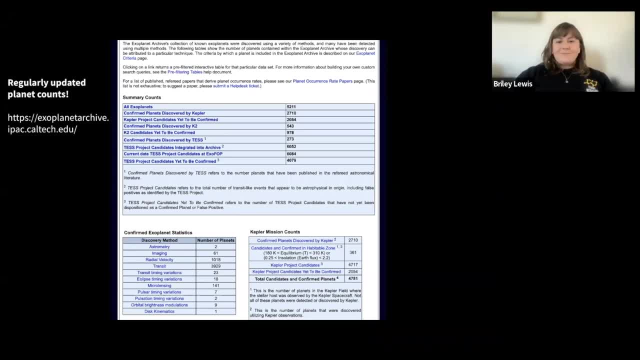 But only around 50 to 60 with imaging. So yeah, definitely go check up on this number if you're ever interested. Someone asked the question: it's hard to see the planet. How would you see a space station? We wouldn't yet really, This was more of a fun. let's imagine if we could find everything. what would? what would you be excited about? question, So that we would have to have a lot, a lot, you know, more advanced technology to see something like that. 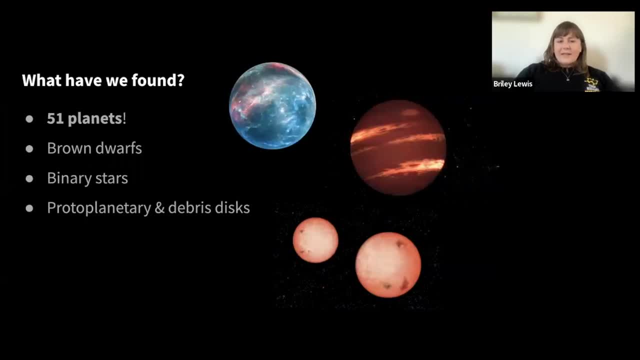 All right, so back to what have we found. So we'll get to the planets in a little bit. But what about these brown dwarfs? Those are some things that you know. I think some people might not know about. Why are they cool? What are they? 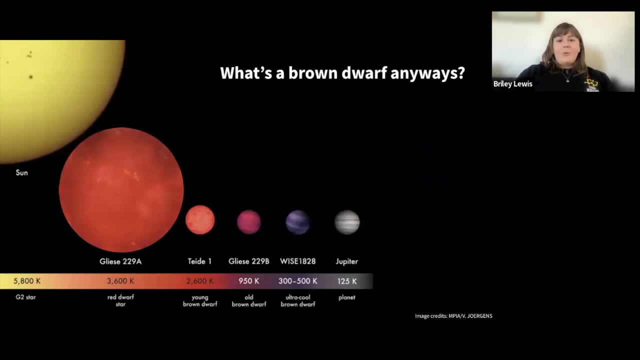 So what's a brown dwarf anyways? A brown dwarf is something that is between the mass of the biggest planets and the smallest stars. So here you can see the sun compared to a red dwarf, the smallest kind of star. Then there's three different brown dwarfs that are between the mass of that star and Jupiter. 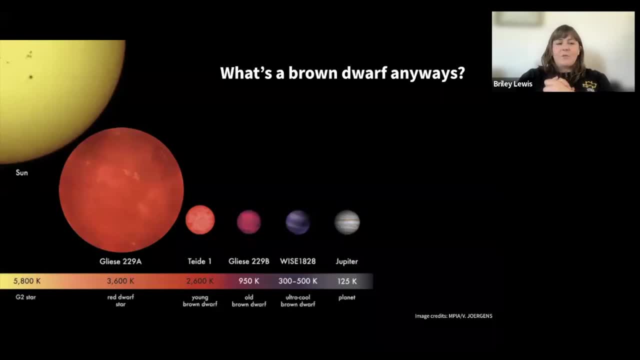 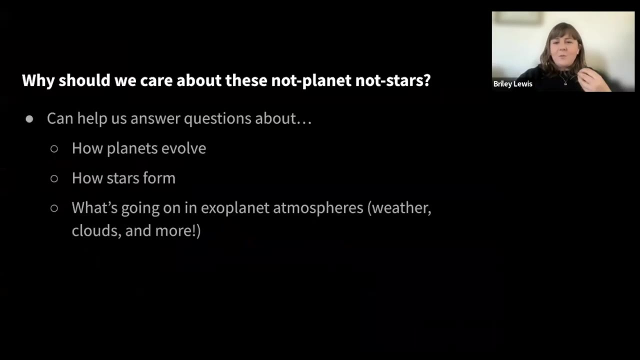 And so these little in between things. some people call them failed stars because they never actually ignited hydrogen to helium fusion to make them burn bright like stars do. I don't think that's quite right. They are these weird in between, So why should we care about them? Because they can help us answer questions about sort of what. what's the difference between forming a big planet like Jupiter? 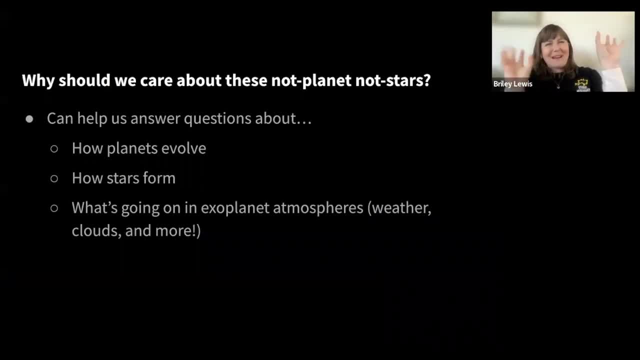 And what's the difference? Sorry, what's the difference between forming a big planet like Jupiter and forming a full on star? And because they're, you know, bigger and brighter than Jupiter and therefore easier to see, they can help us start to answer questions about how planets evolve and what's going on in exoplanet atmospheres, because it's easier to see their atmospheres than it is to see Jupiter. but we think they have a lot in common. 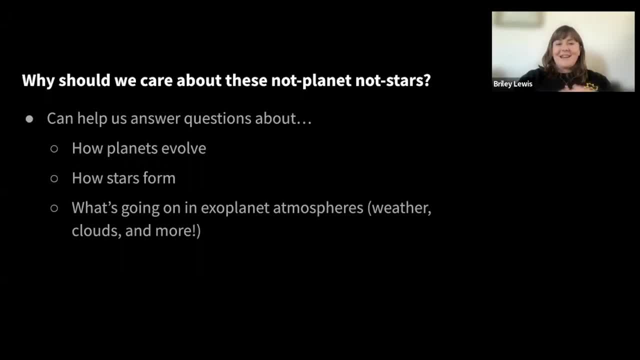 So we look at brown dwarfs to try and get an idea of You know how these different things form and also what the atmospheric- like chemistry and motion and stuff like that- is for a big, you know ball of gas. I've got a couple questions I'll answer real quick. 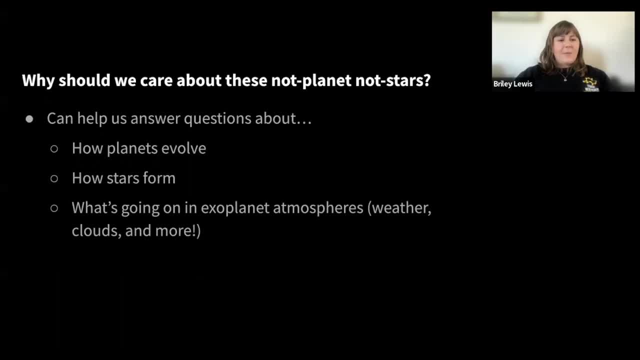 Someone says there's a long list of potentially habitable exoplanets, but which exoplanet is most promising? I don't feel like I can answer that yet. I don't think we have enough information. So the hope is that, with you know new telescopes like JWST and others. 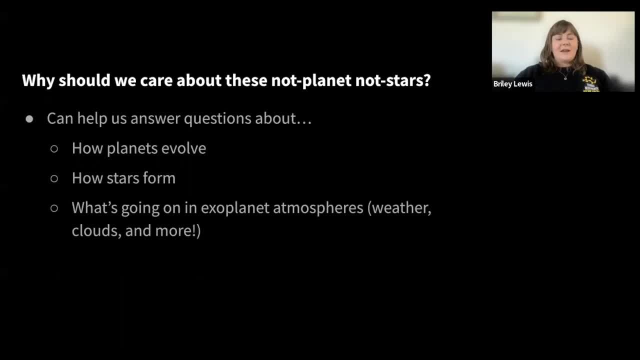 But with other upcoming telescopes like Roman, and then eventually it used to be known as LUVEX. Now people kind of call it Civic Becks or reasons I'll get into a little later. So upcoming telescopes will hopefully be able to actually show us some biosignatures and you know where our four. we will have a better idea of which one is a good candidate for life. 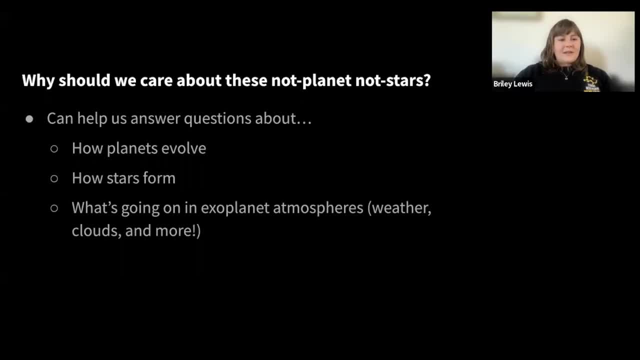 The question in the chat was: Let's see, Let's see different galaxies that are like the same as ours, um, and so, to be clear, when we're talking about exoplanets, we have only found exoplanets within our galaxy so far, um, with the exception of a. 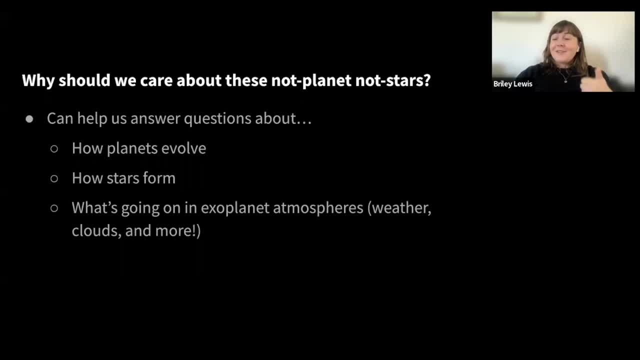 couple maybes from like microlensing and stuff, i think. but as far as transits, radial velocities and direct imaging, we are only looking- and actually are very close by neighborhood- because further away we can't. we can't see that yet. um, because the planets are just too small and too. 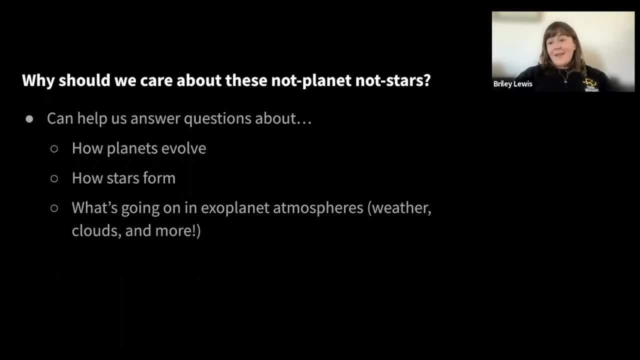 faint, um, but from everything we know, there's no reason that planets like ours shouldn't form around other stars. um, it formed here. um, for all we know, life could be a really common process that happens in the universe. so what we're going to do now is we're going to go on a little tour of. 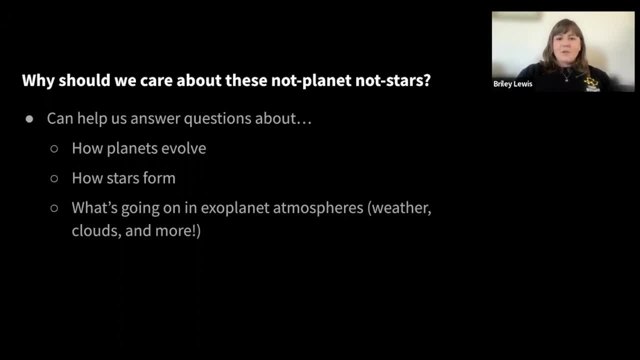 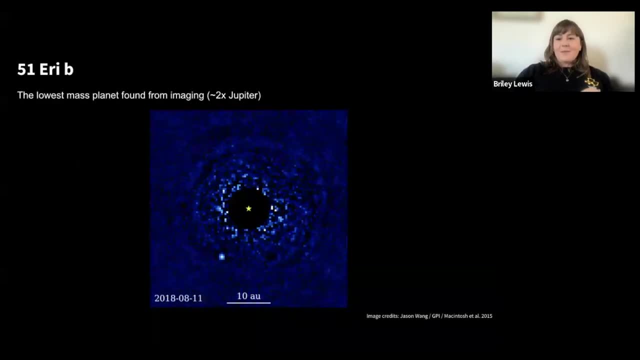 a couple of the discoveries from direct imaging. so let's move on to our first one. this is 51 era, the, the. this is the lowest mass planet that we've found from imaging. so it's two times the size of jupiter and you can see in this image that we actually can see some of its orbit. so what we're going to do in? 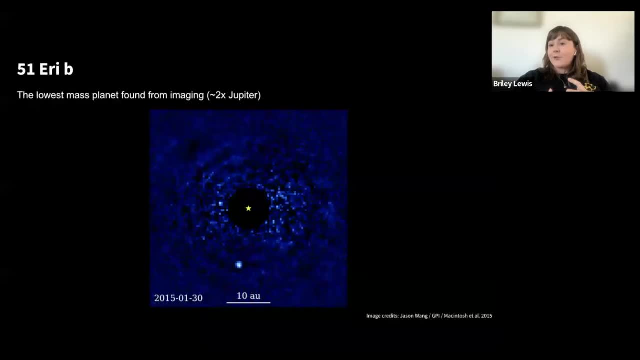 this bit is. i'll tell you about one of the discoveries and then show you the telescope and instrument that actually made it so. 51 eridani b is currently our record holder for the lowest mass image planet and hopefully we will break this record soon. and this one was discovered with the 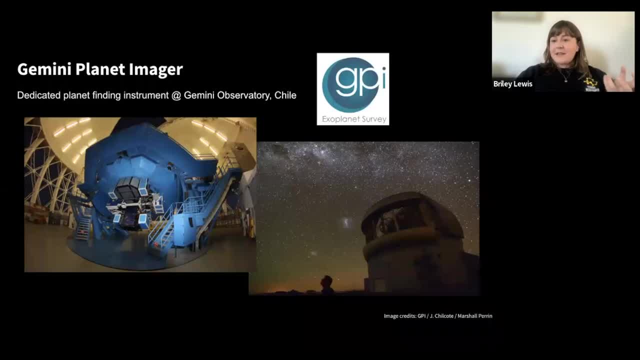 gemini planet and it's a very famous planet and it's a very famous planet and it's a very famous planet imager. so this was a an instrument for the telescope that was, you know, dedicated specifically to planet finding. that is what it was designed for and it used to be on the gemini south observatory. 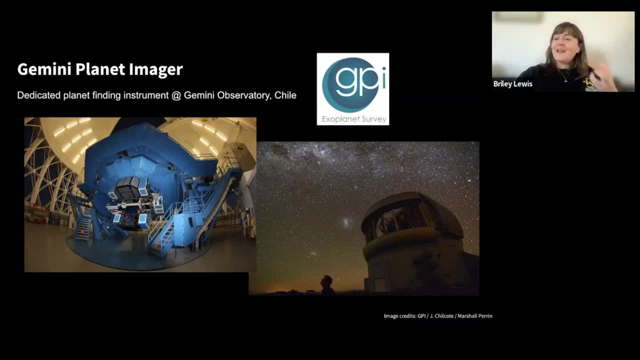 in chile, and now the instrument has actually been taken off the telescope and shipped back up here to the us, where the gemini planet imager team is upgrading it and will soon put it on the gemini north telescope in hawaii. since you guys are observers, you probably know you can see a different. 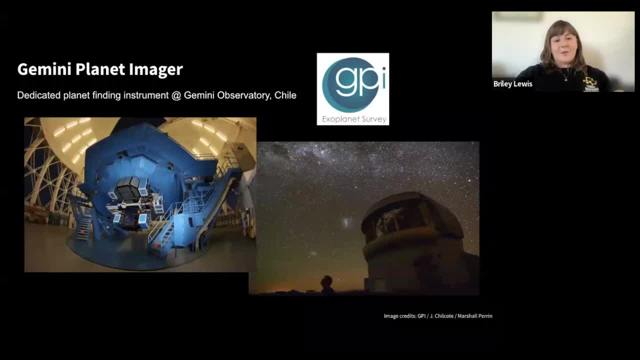 set of stars and you can see a different set of stars. and you can see a different set of stars and you can see a different set of stars in the south than you can in the north. so gemini did a survey of. so gemini did a survey of stars, looking for planets in the south. so, and now the gemini, 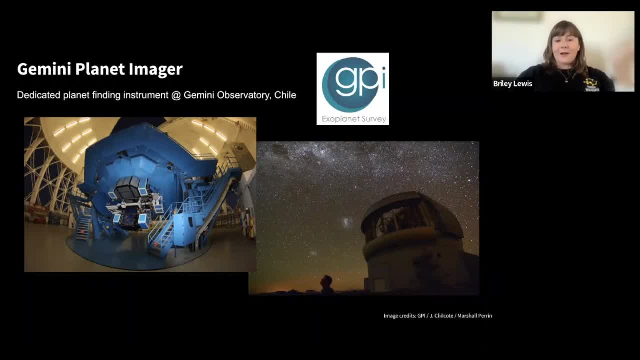 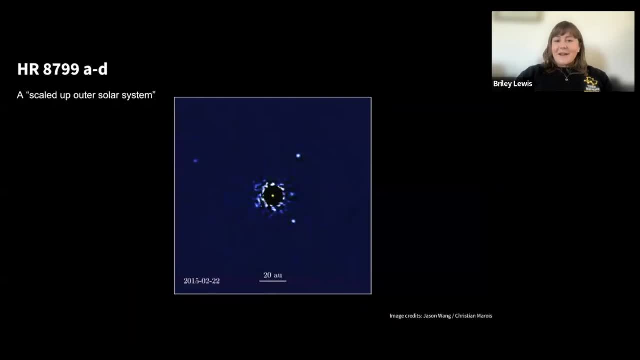 planet imager will hopefully do something similar in the north with an upgraded, bigger, better everything instrument. this is one we looked at already today. so this was our i đâu slide image hr 8799. so a is the star itself and then bcd. uh yeah, bcd and e. i should have said b through. 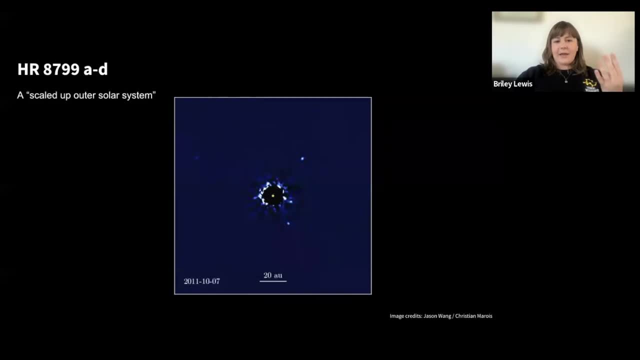 e, not a three e b, not a three e. i should have said b three, three b, not b three e b, not a three through D. So B, C, D and E are the planets. So each of these planets that you see, each dot. 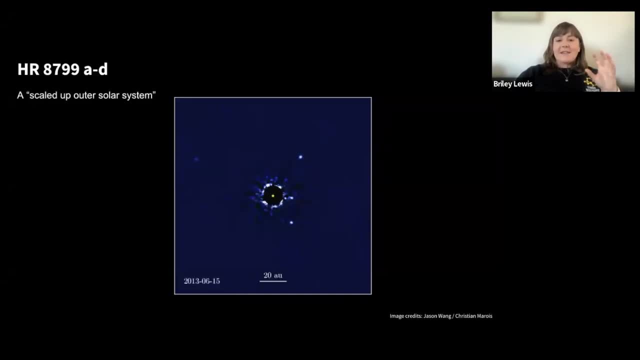 is multiple times the mass of Jupiter and they are double the distances of Jupiter, Saturn, Uranus and Neptune respectively. So this is kind of like a big scaled up version of our outer solar system and it's one of the best studied directly imaged systems You can see based on the time stamps. 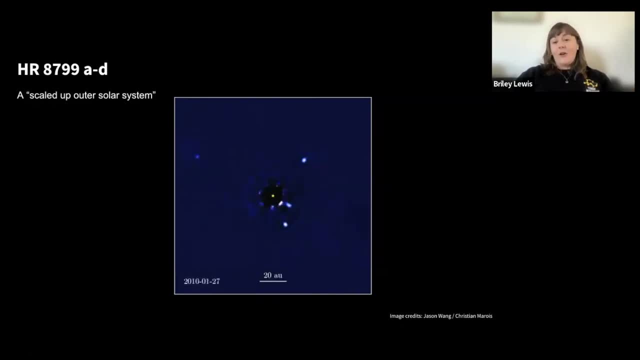 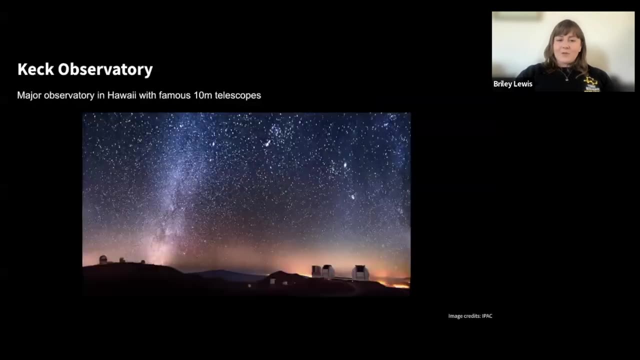 here that we've been observing this for a long time and still are to try to get more information about this system so you can really understand it. And that photo was taken with the Keck Observatory, So this is a major observatory in Hawaii with famous 10 meter telescopes. 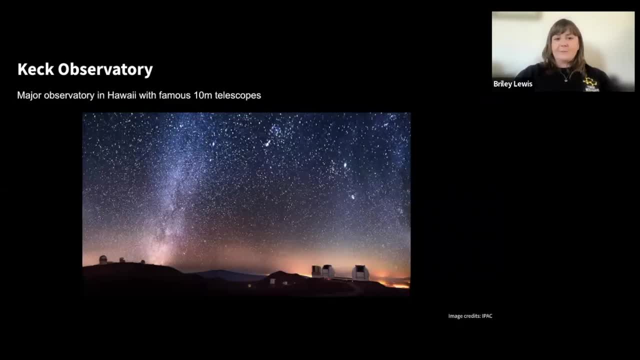 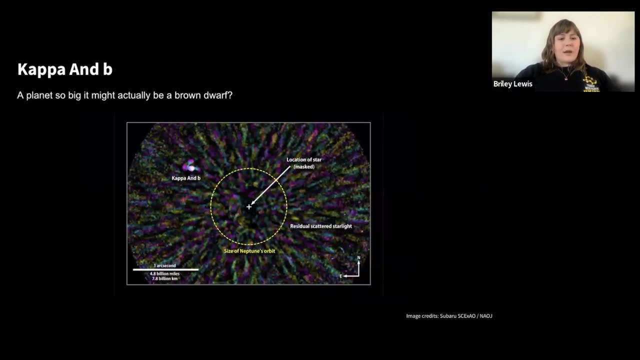 and a lot of different instruments that can be used to investigate planets. Oh, we got a question: Is the adaptive optics in the imager or in the telescope? So it is part of the telescope facility, but does you know work with the instrument, if that makes sense. 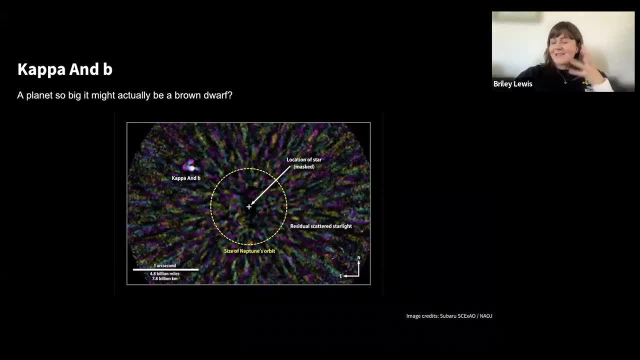 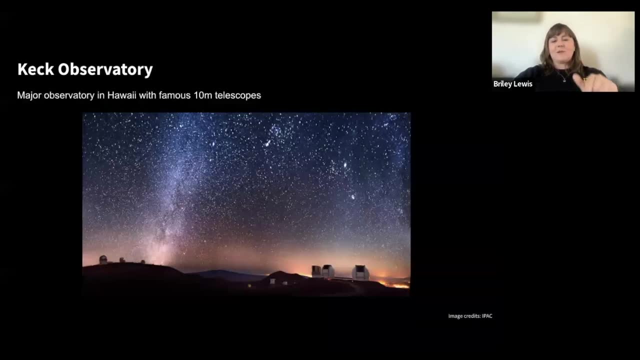 So adaptive optics are a feature of the facilities, like Keck has its adaptive optics system where you can use the laser guide star which you let's see- it's not in this image, but sometimes you'll see images of the Keck telescope like a laser pointing into the sky to record the adaptive. 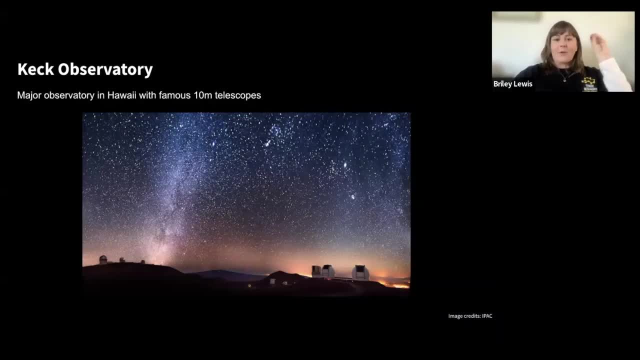 optics system or you can just, like you know, use it on on a star without using the laser. Another question: How far away is the farthest star with an exoplanet that you can directly visualize? And I don't actually know that number off the top of my head. 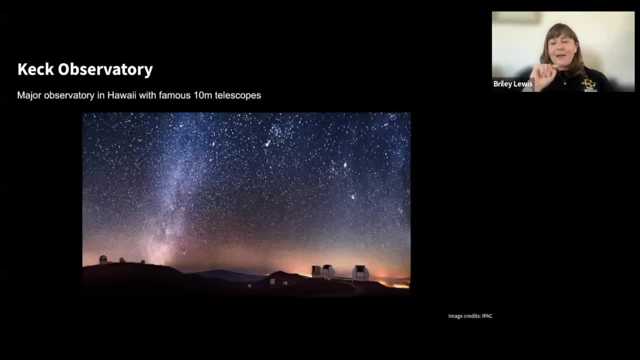 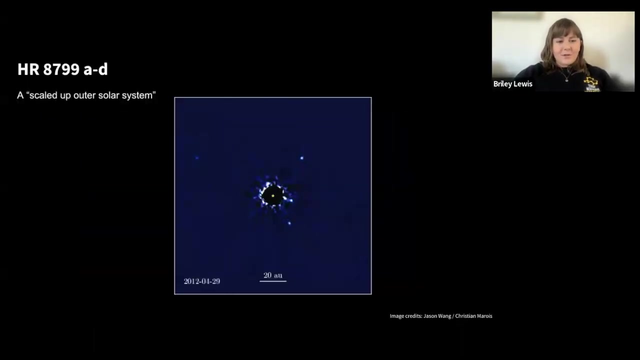 It's not that far. So if you were to draw a picture of our milky way and you know where our sun is out, on one of the arms, the the dot is is very, very small. We are not seeing a large fraction of our milky way. Another person asks: what were the circular? 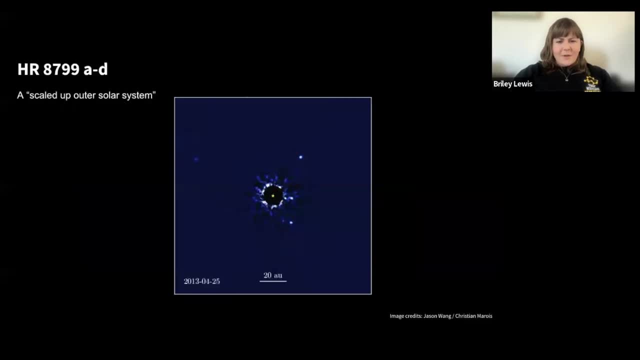 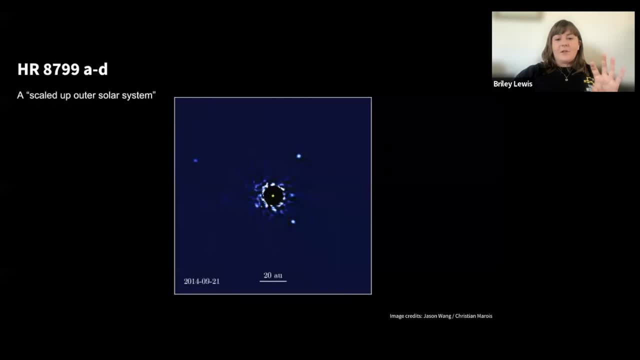 So the center is right where we've blocked out the star and all that's happening around the center is a little bit of light getting around that coronagraph from the star. So that's why anything that's right up against where we block out the star 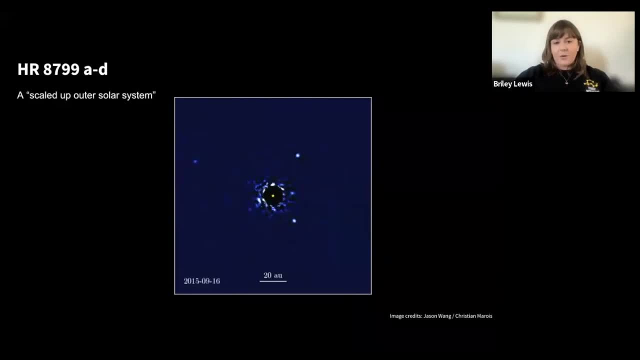 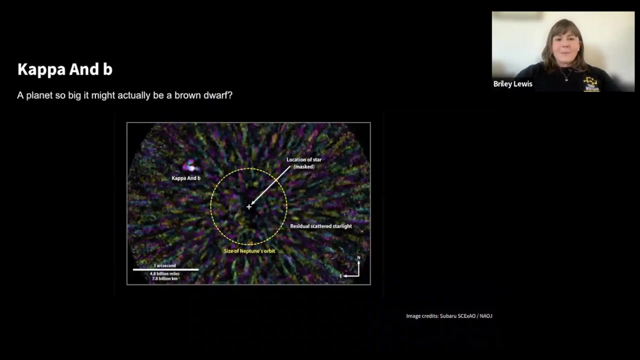 that's why it would be so hard to see a planet there, because the starlight is still getting free. So those, if you're talking about the circular flashes in the center, that's what it is. Okay, so HR 8799. our next one is Kappa Andromeda B. So this is a planet so big that it could. 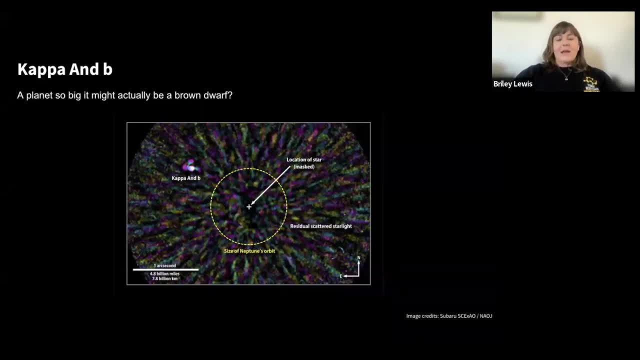 actually be a brown dwarf. maybe People have found out that it's 13 Jupiter masses which is right on the borderline of what we define as a planet versus a brown dwarf. So it's interesting because it's helping us probe sort of that difference between these two categories And 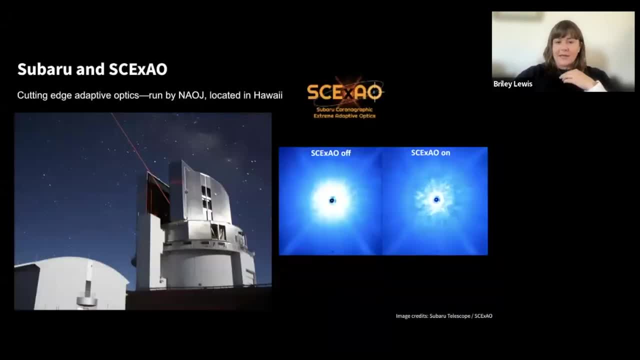 this one was found by the Subaru Telescope telescope, which is also on Mauna Kea and has a really cutting-edge adaptive optics system called SkekSEO, And so on the right here you can see a picture of a star, where the star is blocked out without SkekSEO helping, and then with it helping, So it really helps. 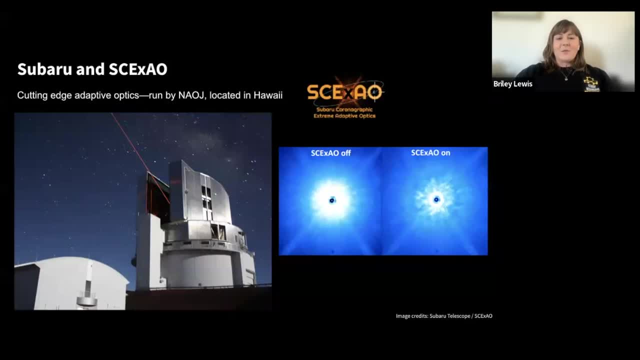 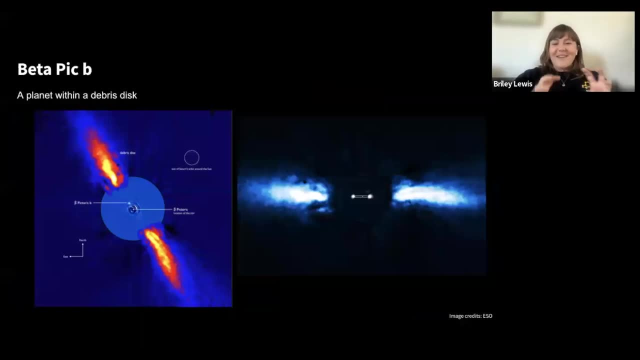 get rid of more of that starlight. And this is a telescope that's run by the National Astronomical Observatories of Japan, And now we're on to not just planets but also disks, So that dusty stuff that someone mentioned in the question earlier. So Beta Pic Taurus. 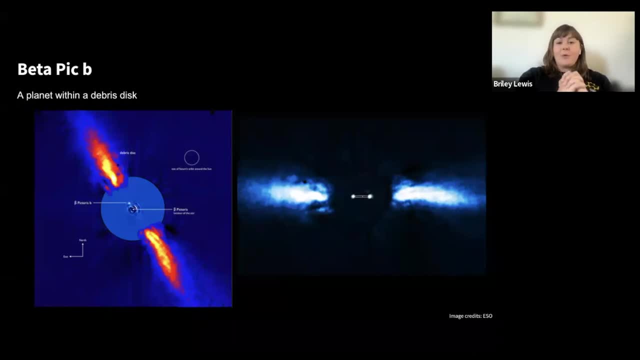 b is this really interesting system where we have seen both a planet and a debris disk, so all of the dust left over from forming planets. So the yellow, red and blue on the outside, that is the debris disk and that's overlaid on a directly image or an image of 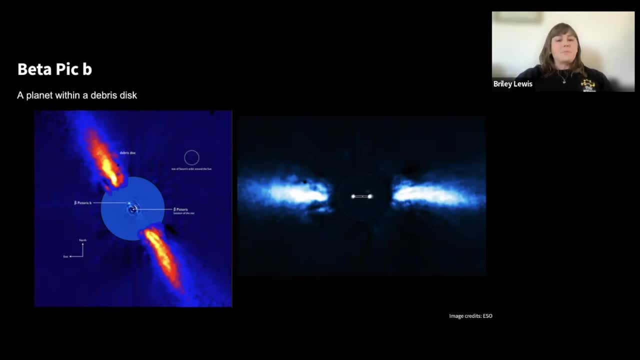 directly imaging the exoplanet Beta, Pic b. So pick these about the orbit of Saturn and we can see- we've actually seen it orbit on both sides of the star, So we've seen that it is edge on a line to us, basically, and it's orbiting back and 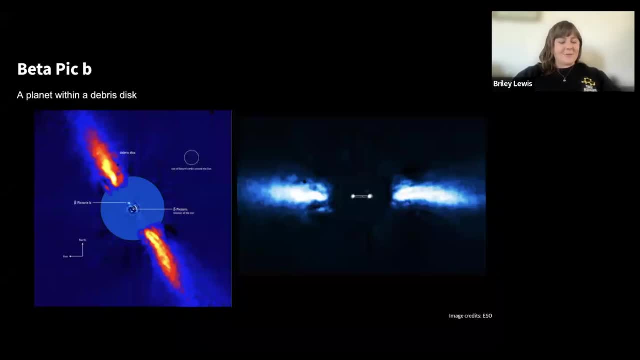 forth. So the picture on the right is the back and forth. Got some more questions. Have we direct image to exoplanets yet where the orbital axis is far from our line of sight? I'm not sure what you mean. We've seen both systems worth edge on, like in Betapik, and then closer to face on, like we. 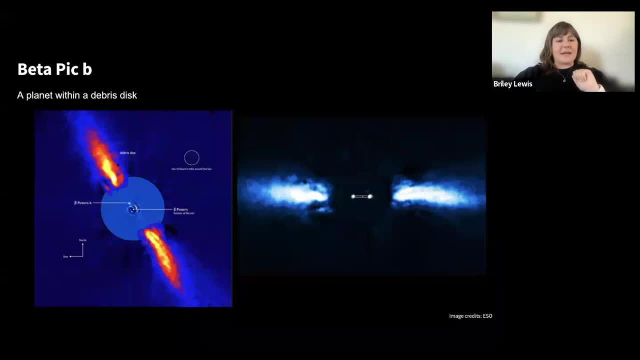 saw in HR 8799.. Then we've got. can a study of the motion of the directly imaged exoplanet through any light show any light on the probable existence of a smaller exoplanet nearby? I don't think anyone's really done that yet. People have done the opposite where you are. 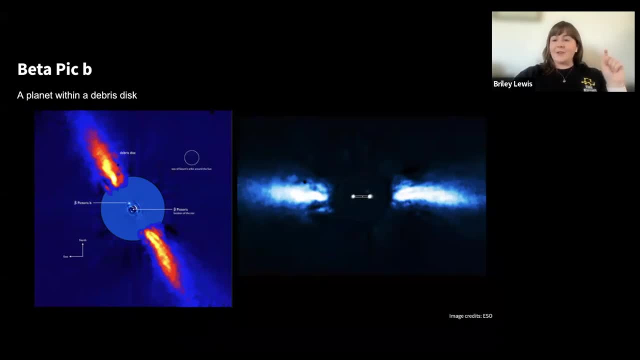 looking at transits or RVs and noticing a signal that shows there might be something far away that is kind of you know, jostling around the smaller inner planet. But I don't know if anyone's done it the other way around. So Betapik B has been imaged by a bunch of different things, One of 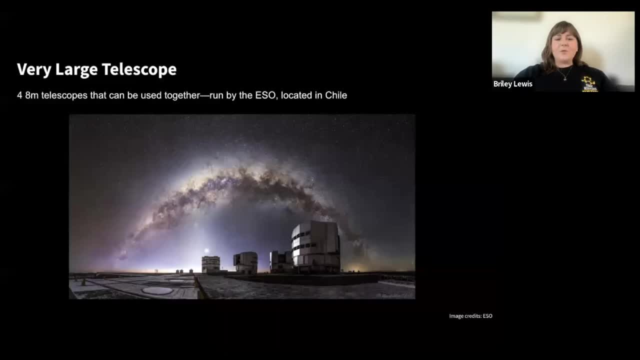 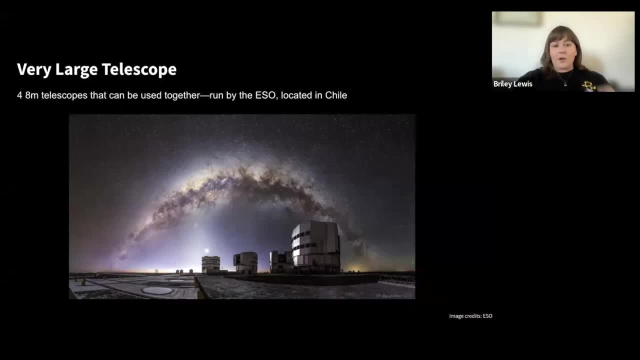 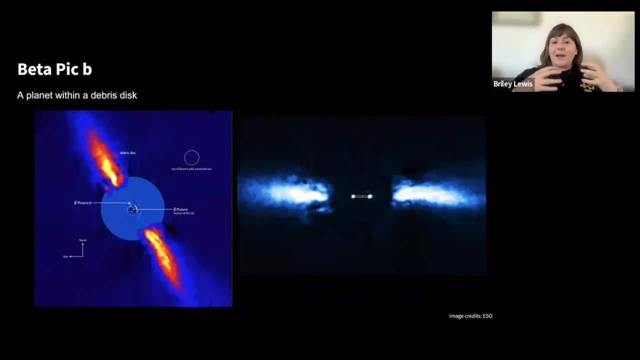 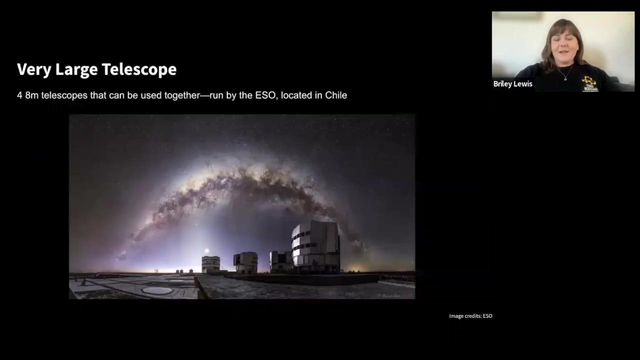 Betapik. And so warps and disks are generally caused by planets, either seen or unseen, you know, moving around that dust and kind of contorting it. So if we see a warped disk but we don't see a planet, it can actually be an indication that there may be a planet hiding from us. All right. 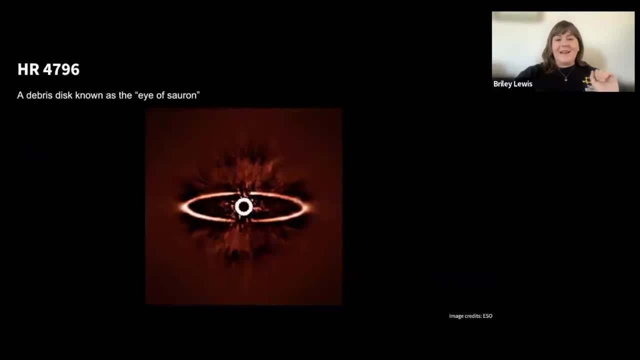 and now a different way to see a warped disk is to look at it from a different angle. So let's look at a debris disk where we don't really see a planet. So the difference between a protoplanetary disk and a debris disk is that a protoplanetary disk is younger, It's the earlier. 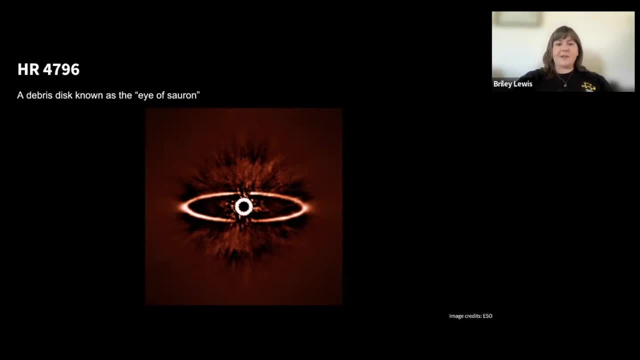 stages of planet formation where there's still a lot of gas around in addition to the dust. But a debris disk is really just dust at that point. It's sort of the elderly planet forming disk. So this is HR 4796.. It's a debris disk known as the Eye of Sauron for, I think, obvious reasons. 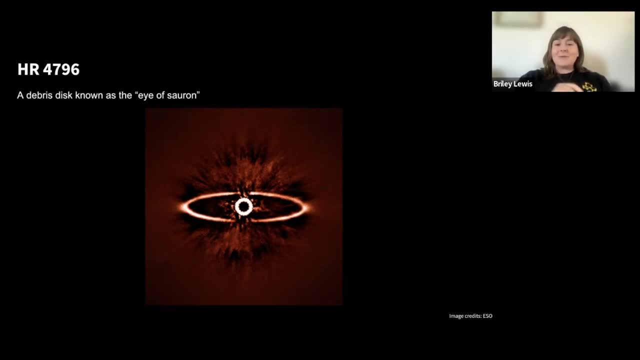 if you've seen Lord of the Rings, If you've seen Lord of the Rings, if you've seen Lord of the Rings, you've seen Lord of the Rings And it's really interesting that we can see this ring of dust. So an analog to this in our own solar system is our Kuiper belt, where we've got a belt of rocky. 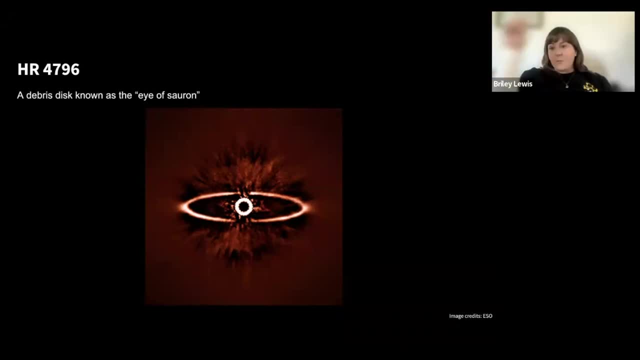 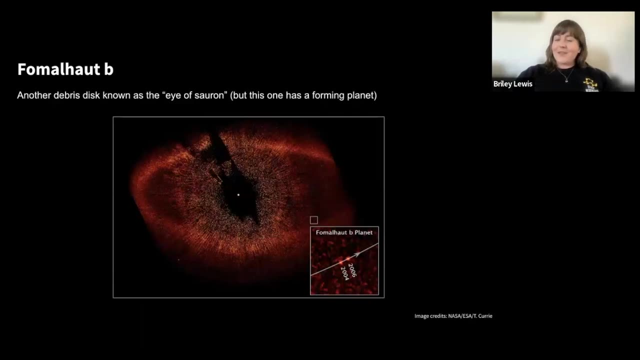 debris, rocky, icy debris that is orbiting, you know, on the edges of our solar system. And then another debris disk known as the Eye of Sauron, because apparently those things just look like this is Fomalhaut and Fomalhaut b. This one actually has, we think, a forming planet in it. 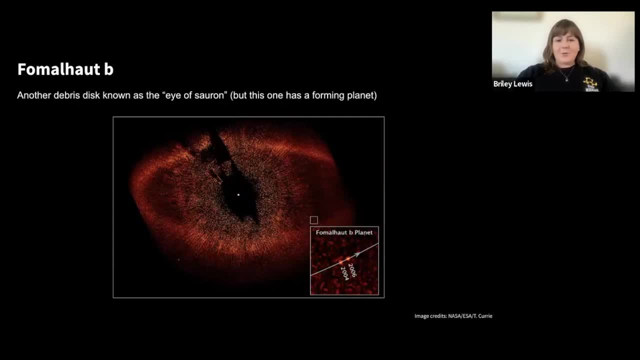 So you can see Fomalhaut's. you know very big, very debris disk here And on this little inset you can see the planet Fomalhaut b. For a while it was unclear if it was actually like a planet. 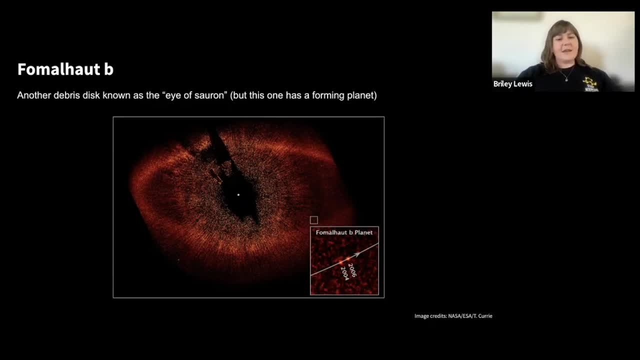 or if it was just a weird clump of dust that wasn't really yet a planet, But it's been observed multiple times moving actually in this disk. And then someone asked what if there's dust getting in the way? Like what, if you know it's a really young system? And the answer to that is PDS 70 b. 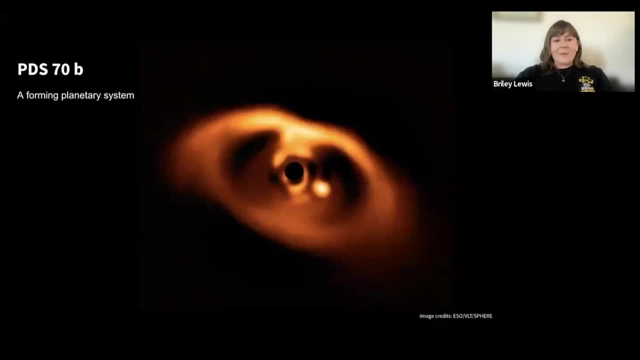 So this is a, you know, an absolute baby planetary system. So you've still got this protoplanetary disk around it And this forming planet that's here, this big lump in the center. you can actually see two little sort of wisps around it as material is, you know. 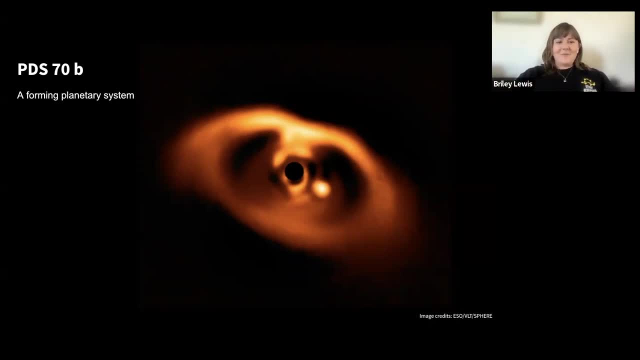 like a preating onto that forming planetary system. So it's time for us to move on. So for our third question. so, Christian, our question time is: which of these discoveries do you find the most interesting? Is it 51 Eridani b, the almost Jupiter-like exoplanet? 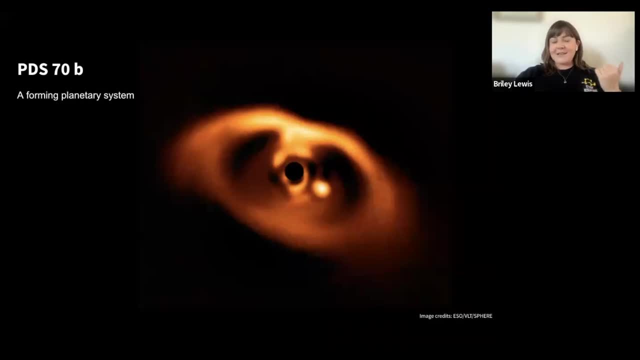 HR 8799 b through d, the multiple planets that we've imaged: Kappa, Andromeda b, the big, almost a brown dwarf. Beta Pic b, the disk that has a planet inside. HR 4796, that thin ring of rocky debris. 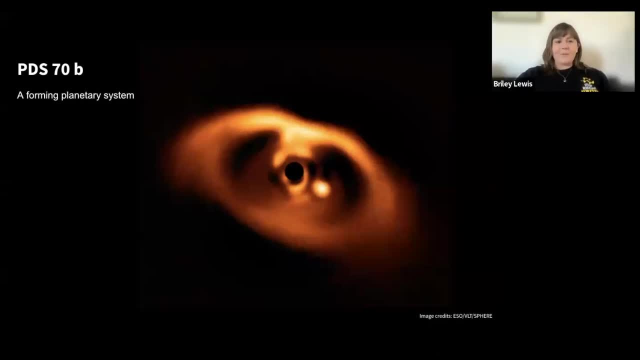 Or this one PDS 70?, PDS 70 b, the baby planet just being born. Yeah, whilst they answer, I can quickly throw in a question. I find the nomenclature so curious here because, you know, for quasars or so. 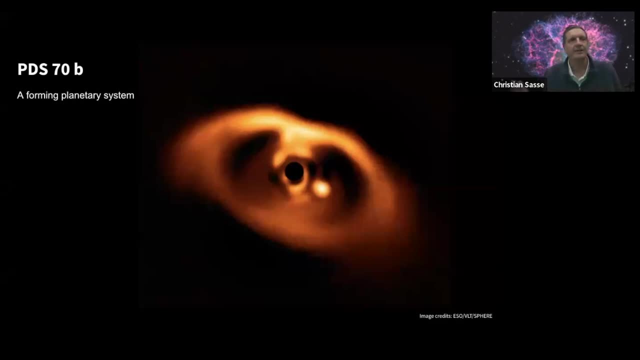 we have a very set, you know right, ascension, detonation, nomenclature. How do they come up with these weird names? Yeah, so the way that exoplanets are named is just after the star that they are around, And so it depends on what catalog they used to identify. 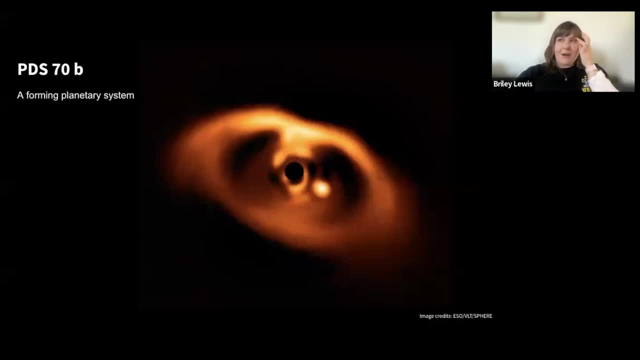 So if you have a star, so HR. oh, I forgot what the HR catalog stands for. A lot of them are HD, which is the Henry Draper catalog. Some of them, the brighter stars, are named So like 51, Eridani is a star in that constellation. 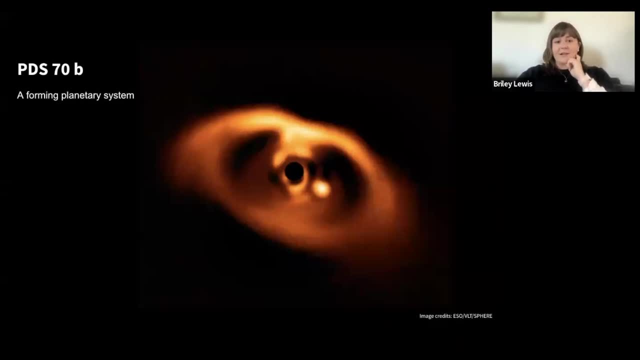 Same with Kappa, Andromeda, that's, you know, a star in the constellation Andromeda, Beta Pictoris, similar thing, And then the others are just different star catalogs that people use to reference, And then the planets are always b? cd. 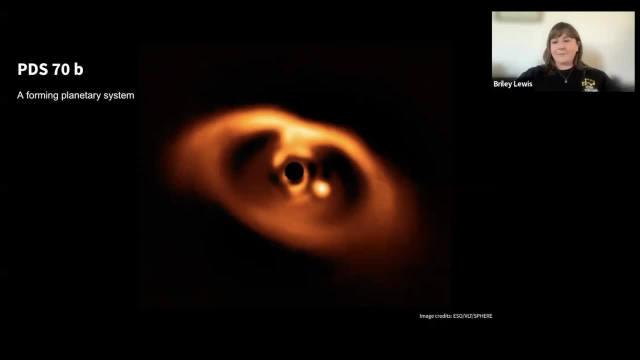 And so on, based on the order that they were discovered. Thank you, That makes sense. Thank you, Yeah, people often ask: if you find an exoplanet, do you get to name it? And the answer is unfortunately no. 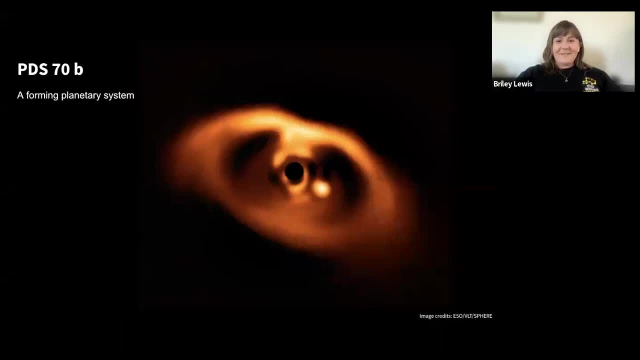 It's really just these numbers. So, oh, we've got a lot of love for HR 8799 and PDS 70b, Close second there by Beta Pic, And then, I think, 51 Eridani b, Kappa And. 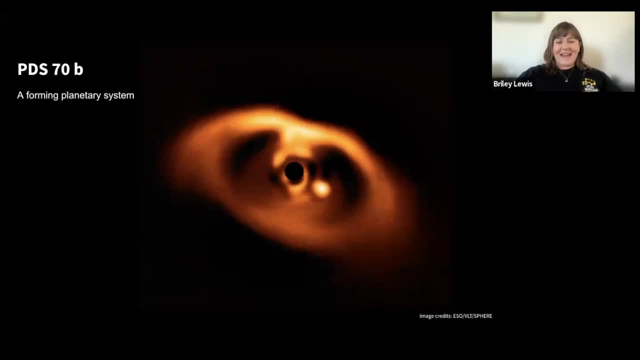 And And HR 4796, they're kind of tied for last year, but still got some votes. I personally think these are all really cool discoveries because they all show us very different things about the diversity of planets outside of our solar system. 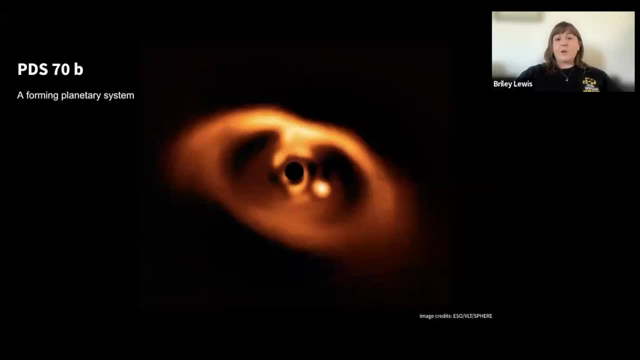 Before we move on, I've got a question. Was the Fomalhaut image visible light? No, these are all infrared. All of the direct imaging stuff I've showed you is infrared. And so what comes next? We've seen some of these discoveries. 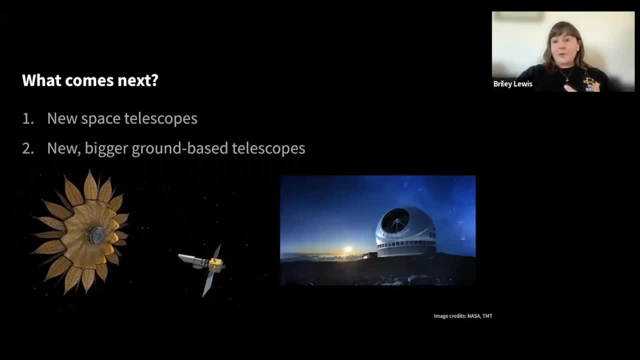 We know we want to see smaller planets, We want to see fainter planets, be able to see them in more detail. So there's really two ways forward. One is new space-based telescopes, because going to space gets us away from that pesky atmosphere, makes that just a non-issue to deal with. 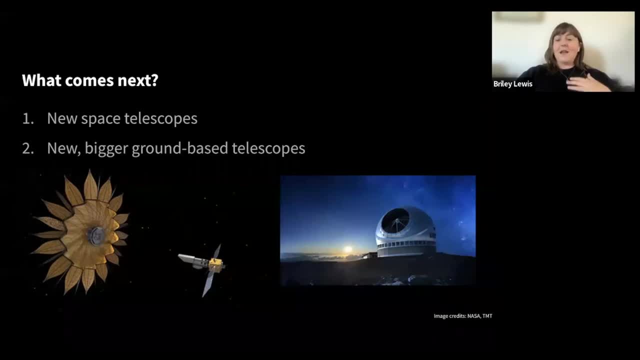 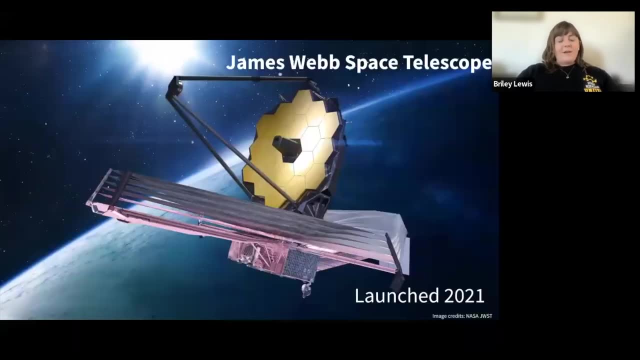 And then the second is new, bigger ground-based telescopes and instruments, because bigger telescopes give us better resolving power to see faint things. So some exciting space missions. One, obviously: the James Webb Space Telescope, launched Christmas Day last year. This has been doing a lot of work. 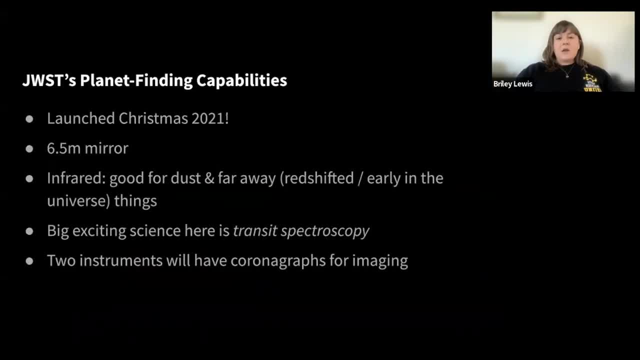 It's been doing lots of cool science all year, So it does have some planet-finding capabilities. This telescope's much bigger than Hubble. It's got a six-and-a-half-meter mirror. It's looking in the infrared, both the near-infrared and the mid-infrared, so longer wavelengths. 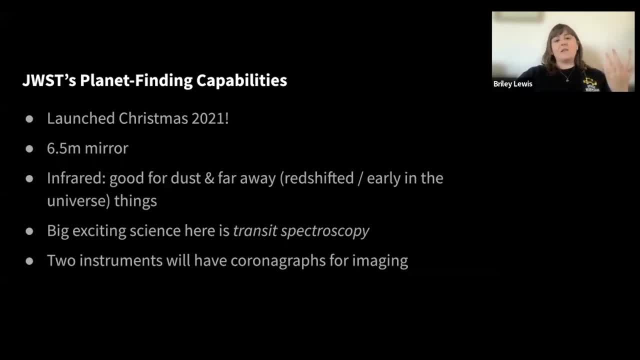 And this is good for dust, which is obviously relevant for planets, and then also far away, like redshifted or earlier in the universe, things which not quite as interesting for us planet folks but cool for science nonetheless. And in the big exciting science, the thing that JWST is really good at is transit spectroscopy. 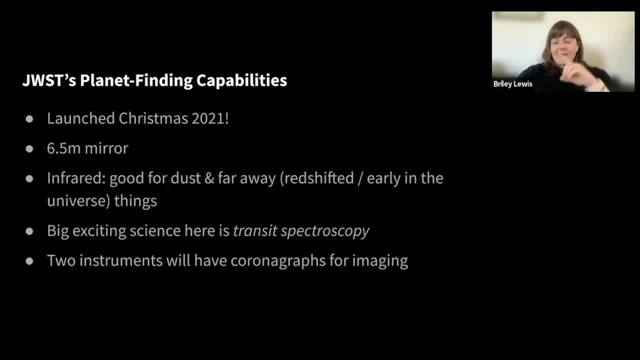 So someone mentioned earlier about transits, how you can actually see the light curves, and transit spectroscopy means you get light curves in different wavelengths and you can use those to figure out where more light is being absorbed by the planet and kind of back out of spectrum. 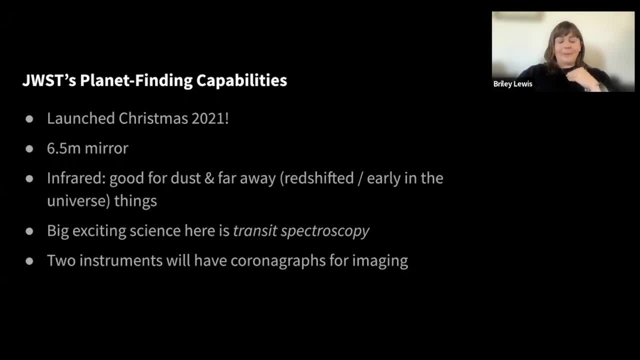 But there are also some instruments that have coronagraphs for imaging, And so two of the really exciting exoplanet results are the one that we're going to talk about today. So the first one is the Hubble Space Telescope, And this is one of the most recent results from JWST so far. 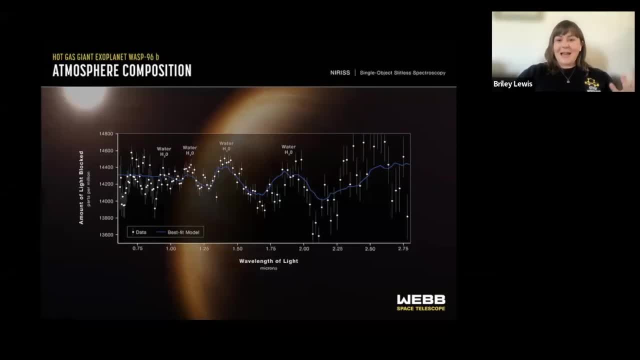 One was released in the first images in July, So this you may have seen in press conferences. This is actually one of those transit spectra. So the enormous mirror of this telescope, along with the precise instruments, made it so that we could actually get detailed measurements of starlight filtering through the atmosphere of a planet outside of our solar system. 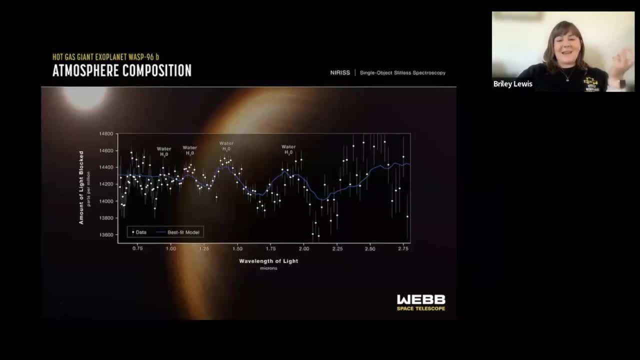 And so this has the information about what's in that planet's atmosphere And has showed evidence of clouds and haze that previous studies of the planet weren't able to detect, because we just didn't have the precision yet. I see a couple questions. I'll answer those real quick. 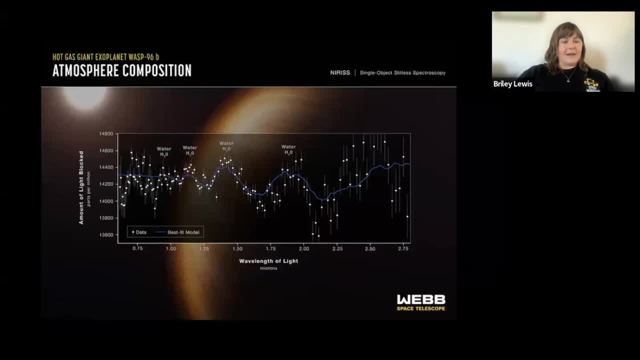 Are most of the exoplanet solar systems similar to the solar system we live in? Is there any known exoplanet which has the possibility to have life or similarities with Earth? The answer to the first bit, no, they are not mostly similar to us. Planetary systems are so much more diverse than what we would have thought Like. there are Tons that look nothing like our solar system and have types of planets we just don't have here And again, like I said earlier, we don't really have enough information to say confidently. 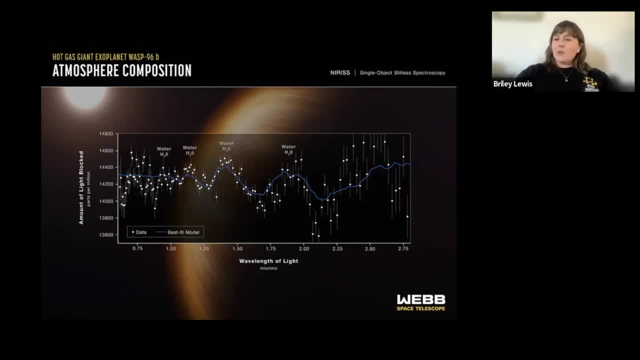 Yeah, this exoplanet, like you know, we think has a good chance of having life. Right now we mostly have. this planet could be at the right temperature for water And that's about the best we have. It's also got. how big does the star have to be for a planet to orbit around it? 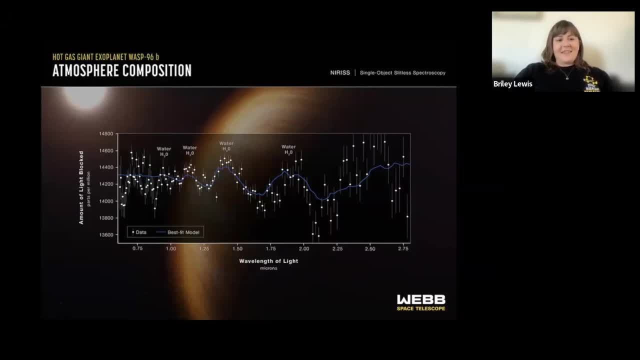 Any of the stars, all of the stars. Things can orbit around. you know, any other thing with mass. So like, even in the solar system we've got binary asteroids, So lots of things, anything with mass can orbit. another thing: 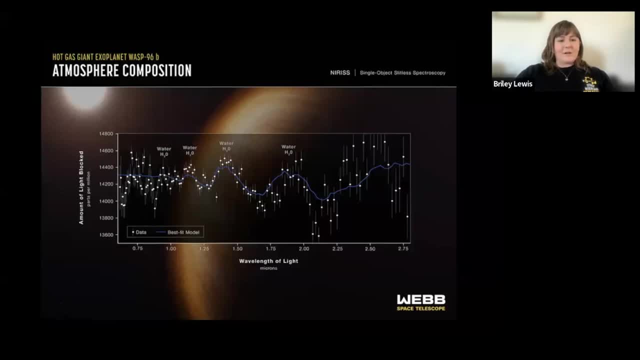 And then just wondering how many directly imaged exoplanets have atmospheric compositions close to our Earth? The answer is zero, because we're only really imaging gas giants right now. We don't yet have the technology to actually image Earth-like planets. So there have been, or I don't think. 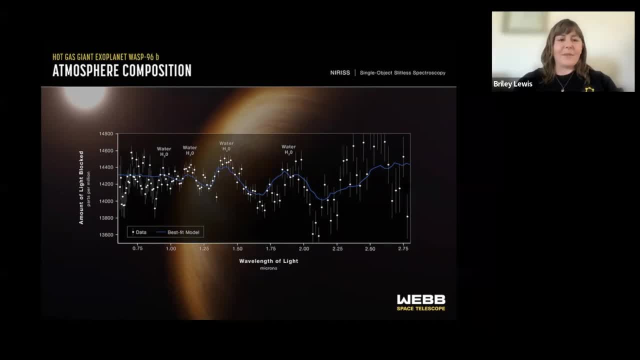 There even have been some with transits like Crespi that have looked Earth-like, But that's because this is really a technique. that's like just you know, we're in the beginnings of this technique And a really exciting time to start getting results soon. 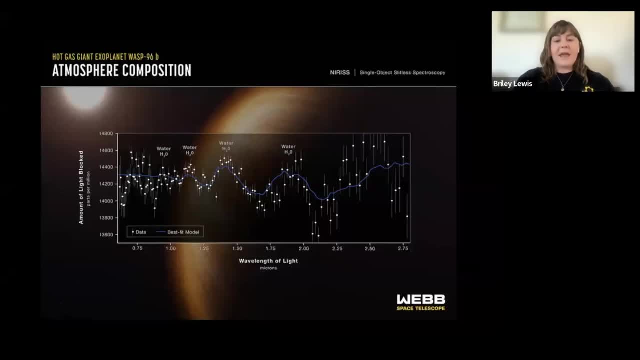 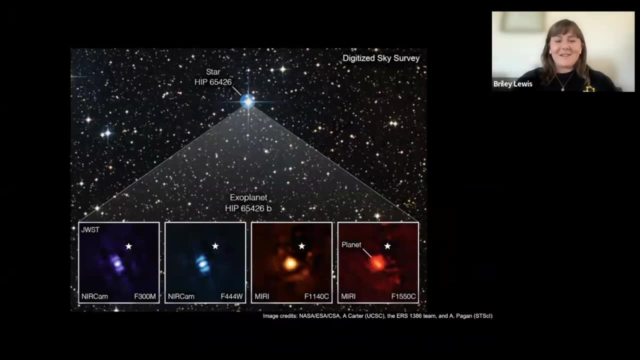 Like this from JWST, And so there's probably a lot more to come there And an image that got a little less press attention. So this is JWST's first directly imaged planet, So around this star it took images in. 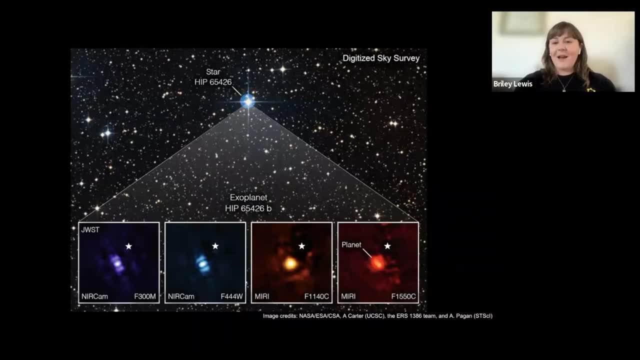 Four different wavelengths of the same planet, And so this is like the most precise spectrum we've gotten of a directly imaged planet so far. You can super clearly see it. It's really awesome and proof that these instruments are working. So this wasn't a new discovery. 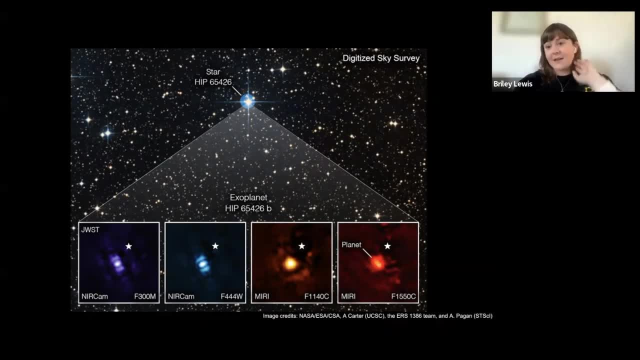 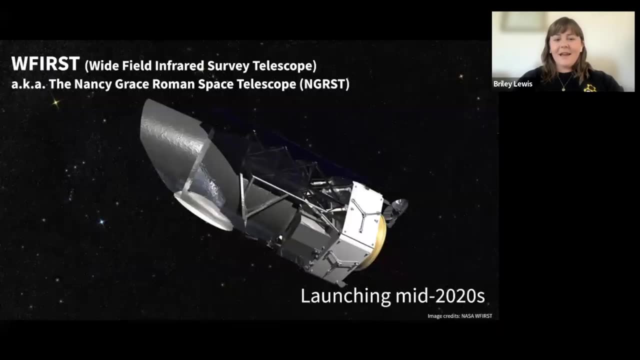 It was an exoplanet we already knew about, but they wanted to use it to test how well JWST could work on- actually, you know, taking data on these systems. Another exciting one: WFIRST, Now known as the Nancy Grace Roman Space Telescope. 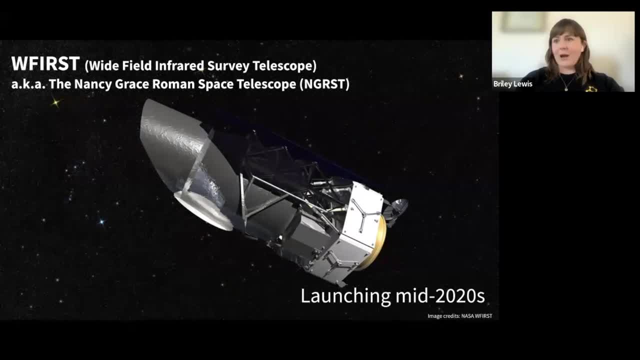 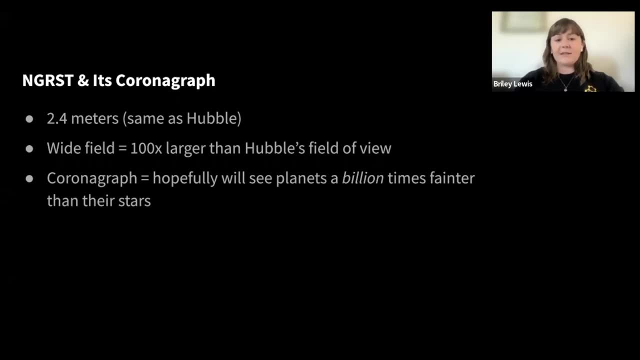 This guy is launching in probably the mid-2020s, which we are rapidly approaching, And NGRSC is going to have a coronagraph, So this telescope is the same size as Hubble, but it's going to have something that's like really dedicated to finding planets. 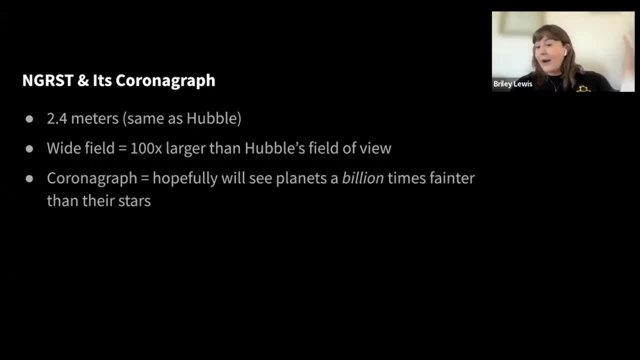 So we call it. you know it was called WFIRST at first because it has a wide field, So its field of view would be 100 times larger than Hubble's, And with its coronagraph we'll hopefully see planets A billion times fainter than their stars. 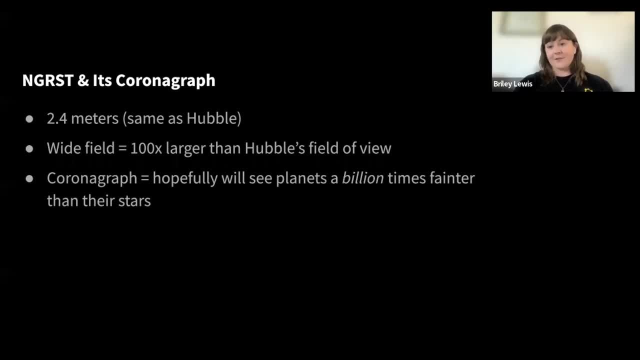 For context, Earth is 10 billion times fainter than our sun, And right now we're seeing planets that are around a million times fainter. So this is a big improvement- not quite all the way to Earth-like planets, but definitely a big improvement. 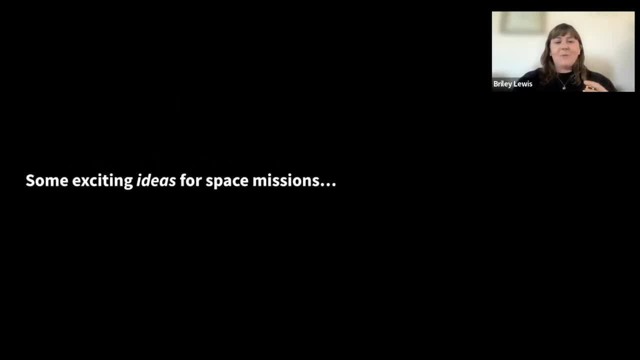 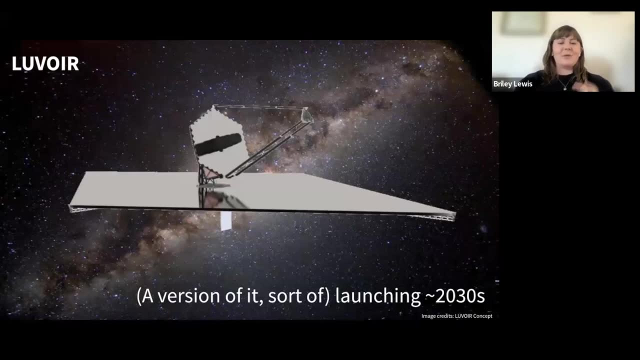 And so there's also some exciting ideas for space missions. So one is the idea of LUVOIR. So I say a version of it sort of, for reasons I'll get into in a second. But so LUVOIR was this idea. 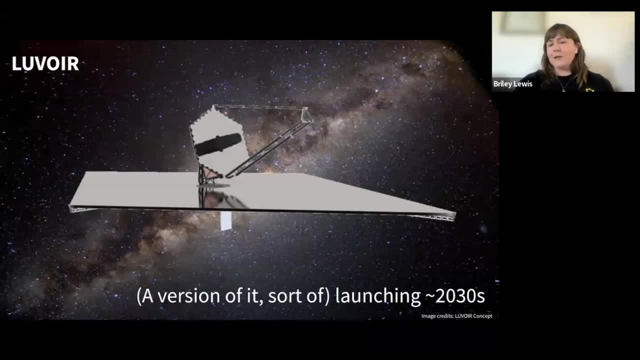 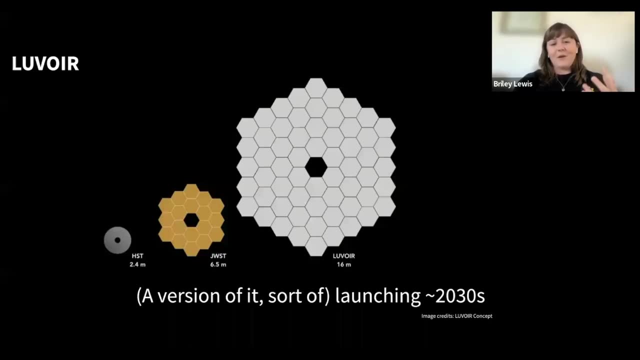 Where people were like let's just make a gigantic telescope like obscenely large. So for comparison, you've got the small circular mirror of Hubble, the mirror of JWST that we think is huge because it's six and a half meters. 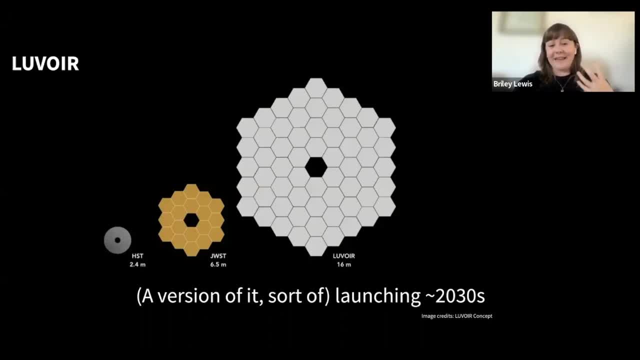 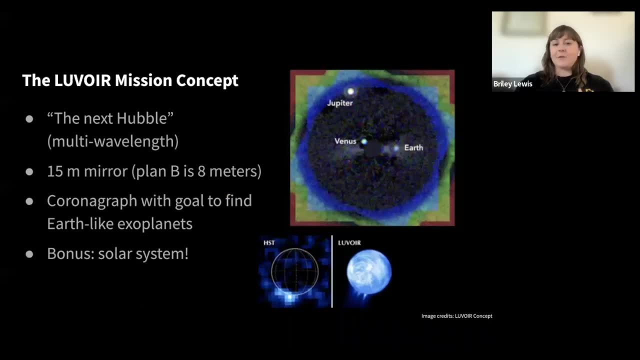 And then the original proposal for LUVOIR was this 16-meter behemoth next to it. So this would be a wild thing if we could make it work And this mission concept considered itself like the next Hubble. So looking at many different wavelengths. 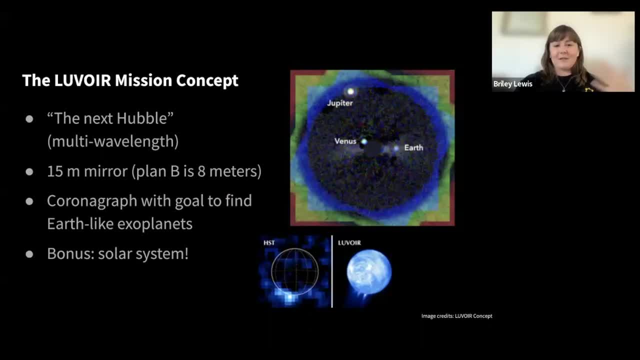 Some like James Webb, which is focusing on the infrared. The original plan was a 15-meter mirror, or there was a plan B with eight meters And it would have. the plan was to have a coronagraph with a goal to find Earth-like exoplanets. 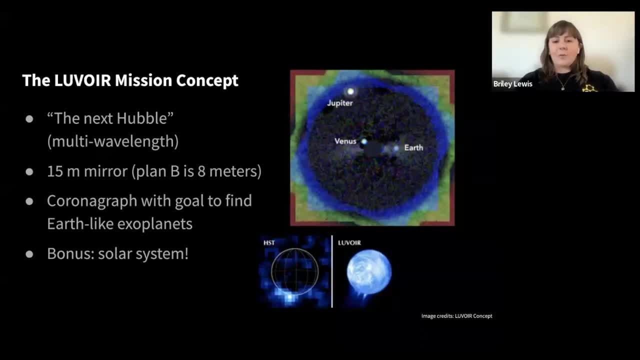 And a bonus, it could do some really cool solar system stuff. So these two on the right are not real data. They are simulations of what LUVOIR should be able to detect. if you know, it was designed and actually created this plan. 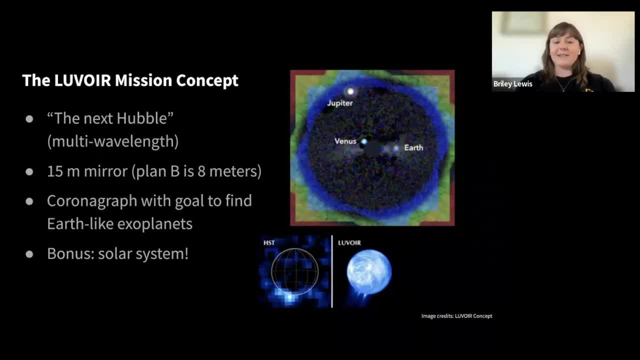 And you can see it would actually be able to image Earth-like exoplanets. And it would be able to do that And it would be able to give us these absolutely wild images of things in the solar system, Like this would be Enceladus with its little water plumes. 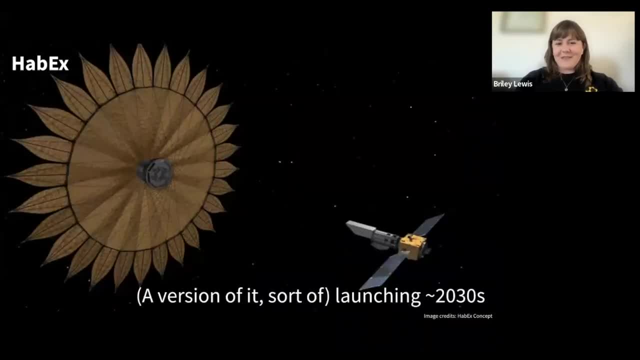 And another one- that is, you know, a version sort of this idea might be launching in the 2030s- is HABEX. So this was an idea for a mission where you had two things orbiting independently of each other but, you know, doing it together. 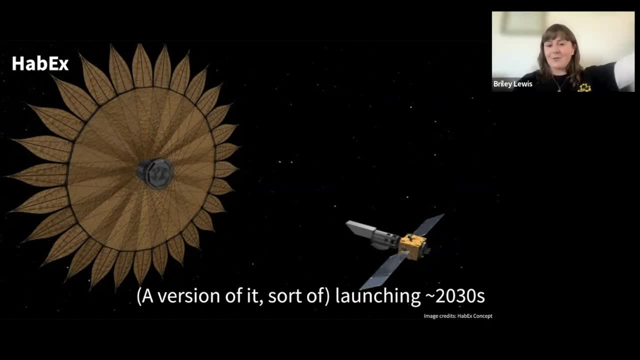 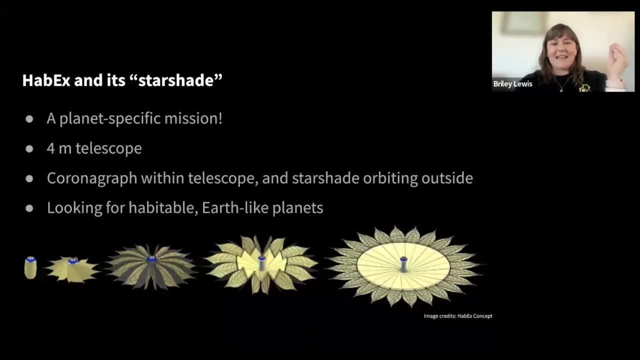 So co-orbiting, where you've got this big star shade that acts as the coronagraph, and then you've got the little spacecraft that actually is the telescope. And something that's really cool is that HABEX would have been just a like. its only purpose would have been planet finding. 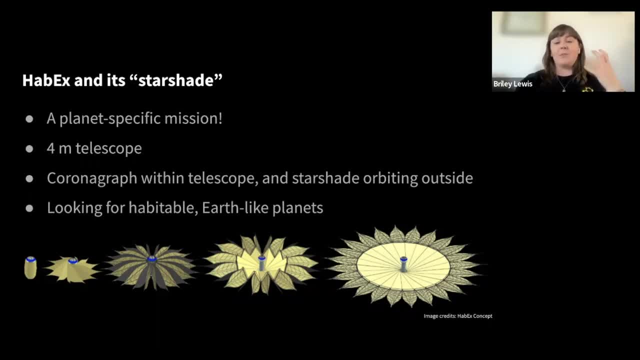 And it would have been a fairly small telescope. but the technology that would have been the really big development was the coronagraph itself. There'd be a coronagraph in the telescope and this star shade that unfolds like this cool piece of origami orbiting outside. 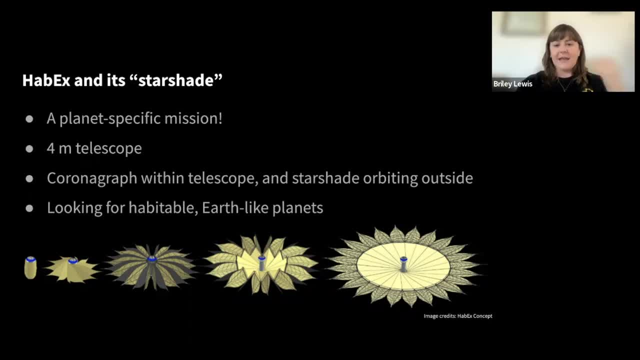 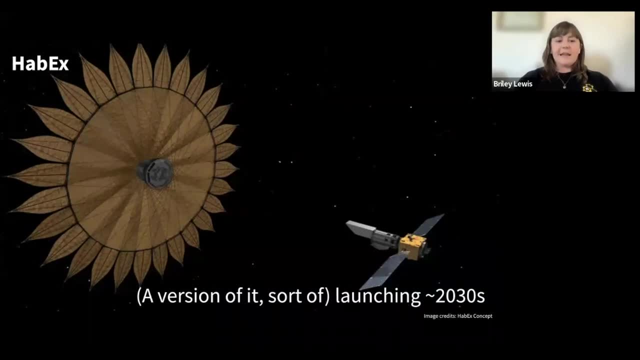 And its goal, HABEX, was to find habitable Earth-like exoplanets, And the reason that I say that for both LUVOIR- A version of it sort of might be launching in the 2030s, is because these were ideas proposed before something called the decadal survey. 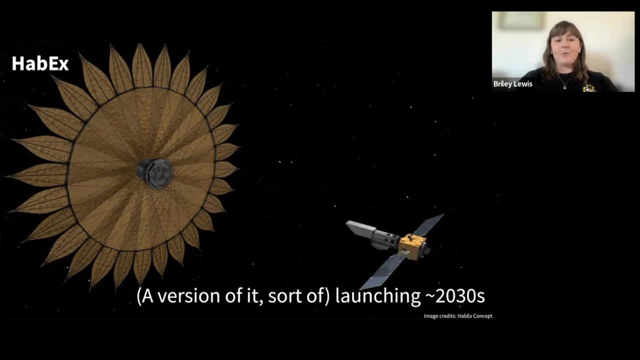 So every 10 years there's the decadal survey, where I see someone says their question is answered, I will miss that one. So every 10 years the decadal survey is a process where astronomers say: here are the things that I think are really important for the field in the next decade. 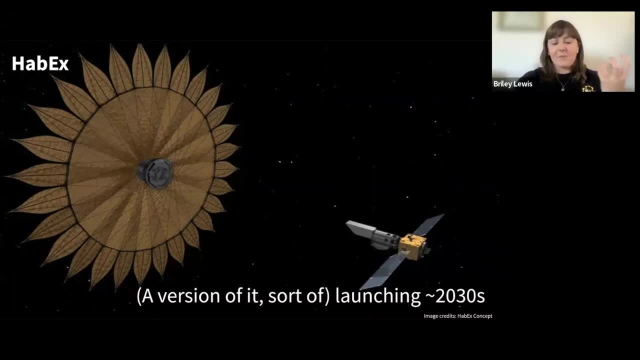 And they write papers and submit them to a committee And then that committee reads through all of the input from the community and helps determine, like okay, here are our recommendations for what is important for the coming decades, And LUVOIR and HABEX were two things that were submitted from the community to be considered as priorities for the next decade. 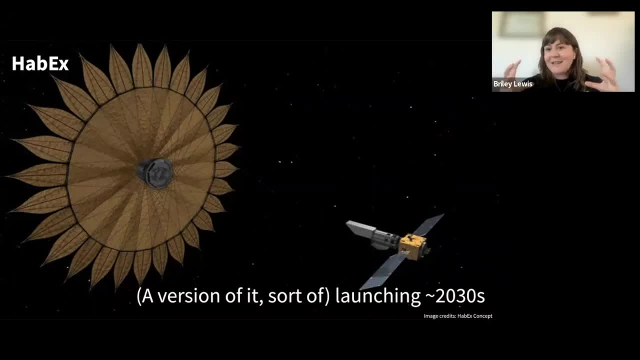 And what the committee came up with was: what if we do a telescope? that's sort of a mashup of the two of them, And so now people informally refer to it as LUVEX- just a combination of the two names. But something like that could hopefully be happening in the 2030s, 2040s. 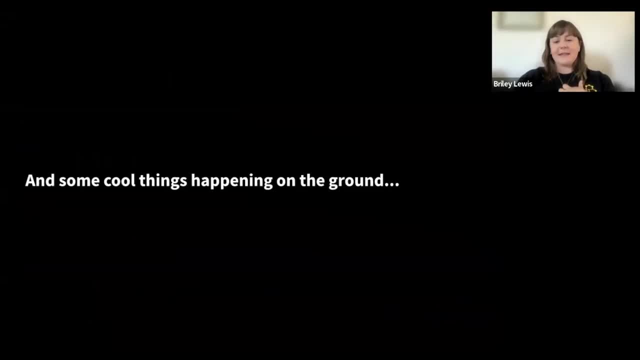 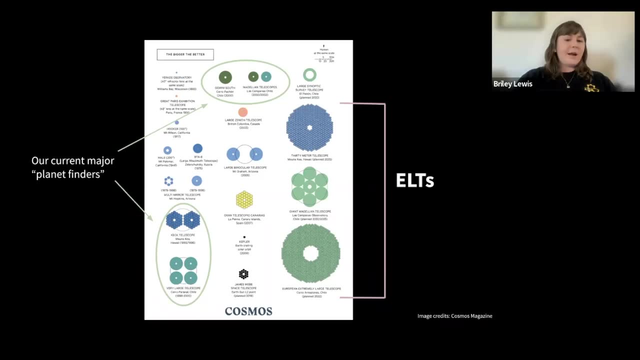 And of course, there are cool things happening here on the ground too. That's what I'm most invested in. So our current major planet finders are circled on this. We've got the Keck telescope and the very large telescope on the bottom that we mentioned earlier, as well as Gemini South and the Magellan telescopes. 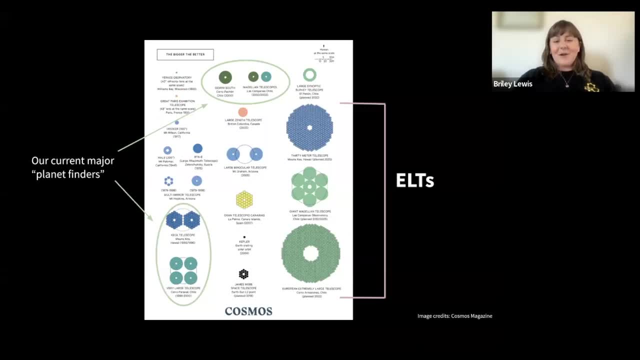 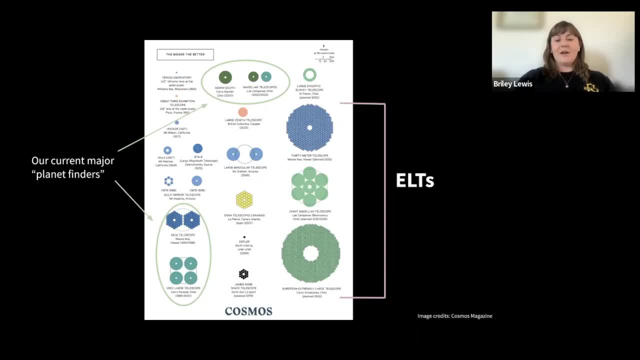 So these are the extremely large telescopes, So these are the sort of next generation of telescopes that are, instead of like a 10-meter across, they're 30 or more meters across, so tens of meters. So remember bigger light bucket fainter thing, as we can see. 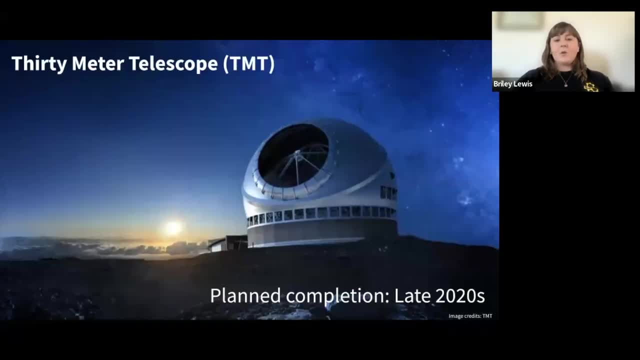 So one of these projects is the 30-meter telescope, or TMT, which was originally planned to be completed in the late 2020s. This is a project that is a partnership between the US, India, China, Japan and Canada. 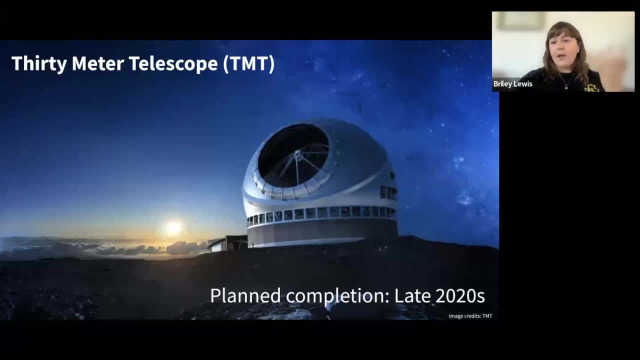 And it's either going to be located on Mauna Kea In Hawaii or in the Canary Islands in Spain. One reason that I say it was originally planned for completion in the late 2020s is that there's been significant debate around where to put this telescope because of pushback from Native Hawaiians over the use of the sacred mountain Mauna Kea. 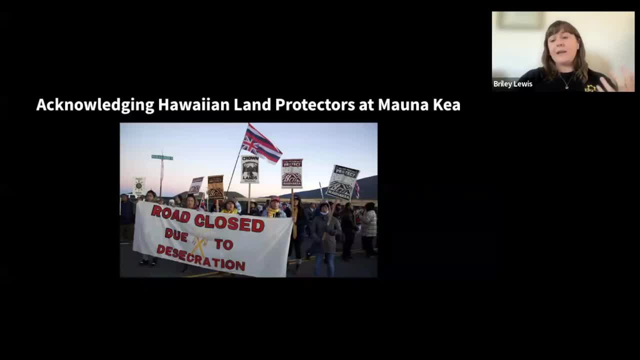 So I want to acknowledge that there are these groups of Hawaiian land protectors at Mauna Kea that are fighting for indigenous rights and this has been a very big conversation within astronomy And you know with kind of how astronomy has been in the news in the last few years, so it's a very complicated situation. I totally encourage you to read up more into it. don't have time to get into the details of it now. unfortunately. 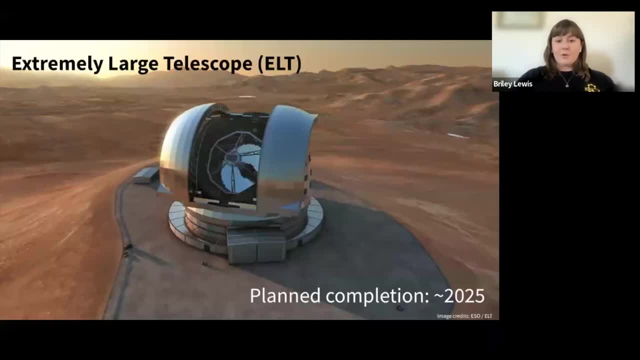 But there are two other extremely large telescope projects that are, you know, still currently going forward. We've got the extremely large telescope. This is the European Observatory's version. It would be located in Chile, in the Atacama Desert, where we already have a lot of telescopes, and is planned to be completed in the next few years, hopefully. 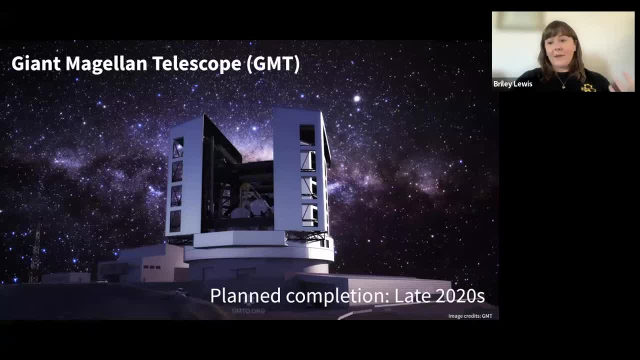 And then there's also the giant Magellan telescope, another one that would be in Chile, And the US does have a hand in this one too. The partners are the US, Australia, Brazil, South Korea, and this one would also be hopefully done at the end of the decade. 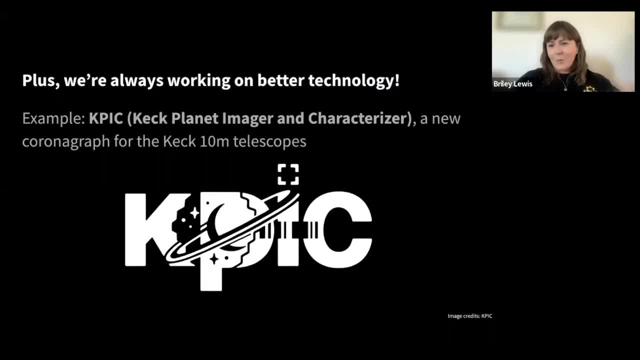 And then, of course, we're also always working on better technology for the telescopes we already have. So at Keck in Hawaii, for example, there's a new instrument that is, you know, currently being developed and tested in- I think just had first light- called the Keck Planet Imager and Characterizer, or KPIC. 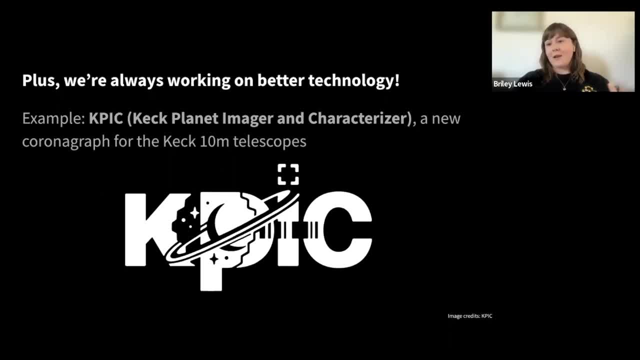 And it's basically a new coronagraph that would help find more planets at Keck. I have a couple of questions I will answer real quick. Someone says: how is radial velocity used to find exoplanets? We're not going to talk about that today, just because that could be a whole other thing, and NASA has a really good website about it. 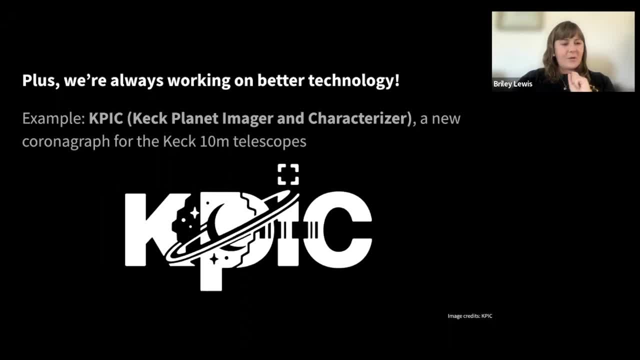 Let's see. does NGRST have a much shorter focal length than Hubble, leading to the capable wide field? And how is the coronagraph working at such shorter wavelengths? So NGRST is also, I'm pretty sure, an infrared telescope. I don't know the details of the design of the telescope itself. unfortunately I'm not really involved with that one. 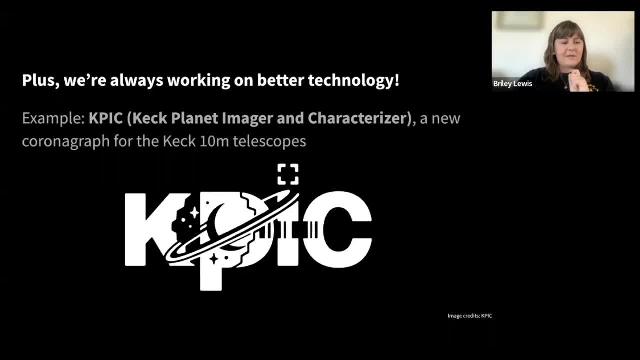 Let's see, since India is also part of this research, as you just told, is there any plan to install an ELT in Ladakh, India, where there are extremely clear skies? I have not heard of any plans to put a telescope in India. 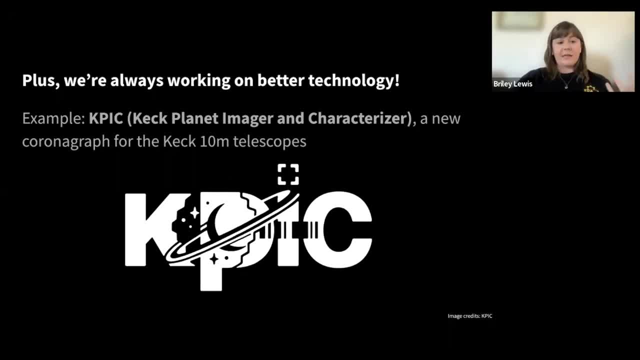 I know we usually put things on Mauna Kea and in Chile, because they are really good conditions where there's not only clear skies but it's also very dry, so that you don't have to deal with weather. And those two places are also very high, so you're past some of the atmosphere and you have to deal with less of it. 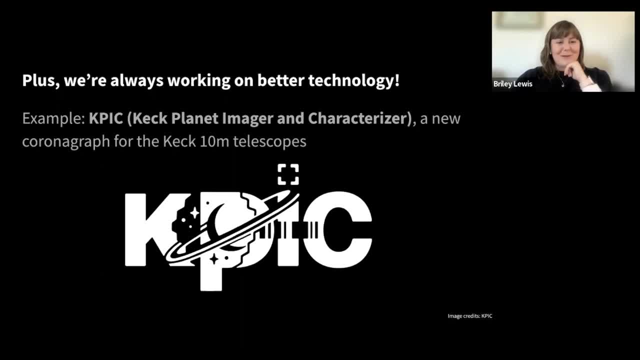 So it's a really interesting suggestion, but I don't know. And then there's another question about tests, which I admittedly have no idea. I have not been keeping up with test news recently, So, yeah, let's move on to the very last bit of this talk.